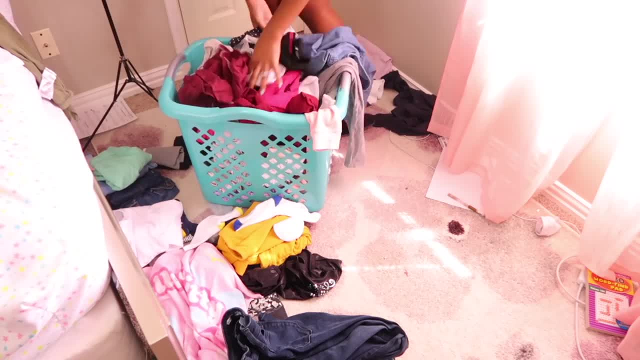 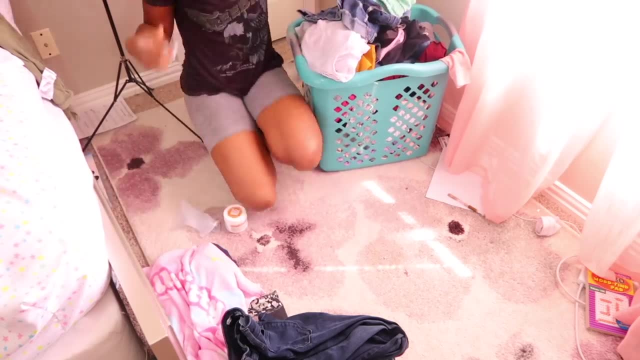 For some reason, being organized and keeping things decluttered is just not something that comes naturally to me, and it does not come naturally to her, So I try not to be too hard on her. Even in my own bedroom things get messy and out of control, but I always take care of it. 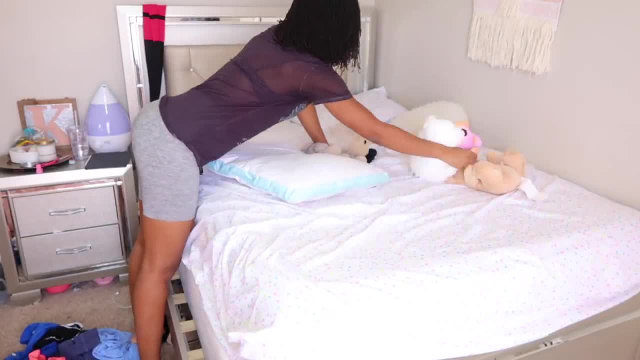 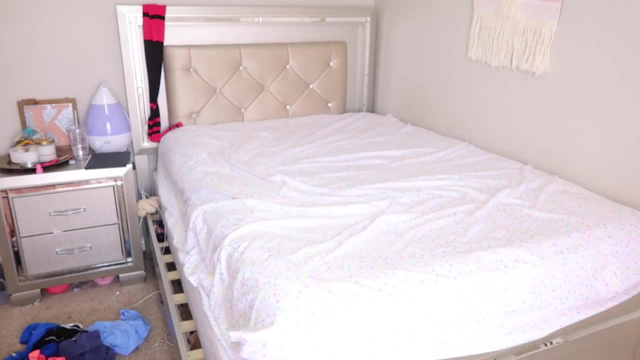 That's the point that I'm trying to get her to. When you see your room get to a certain point of disorder and disarray, that's when you need to kind of take the initiative and start organize some things. at least you know a corner of your room so it just doesn't become complete chaos. 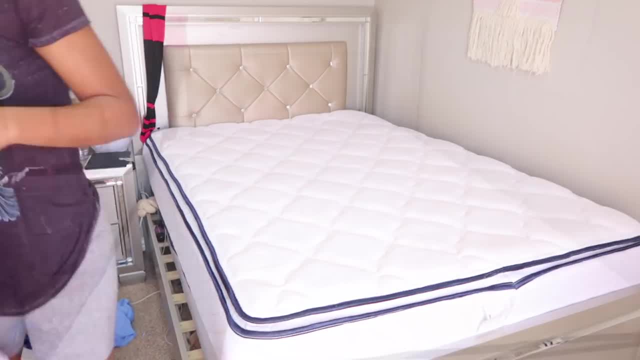 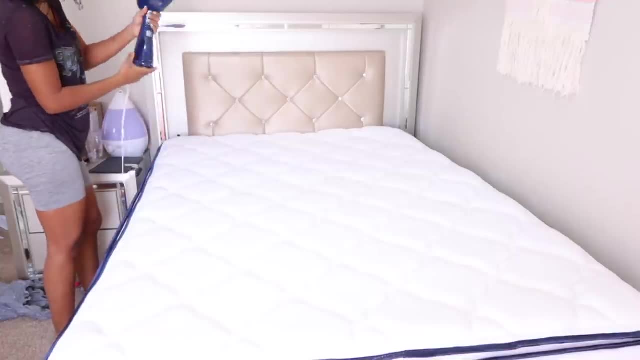 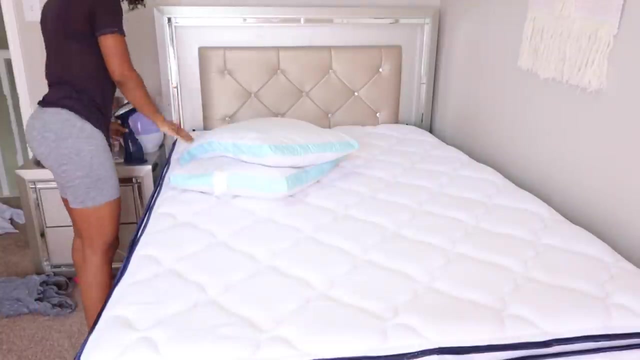 So we're working on that, little by little. So, since I am deep cleaning for spring, I am going to steam clean all of our mattresses and pillows. I already did mine, and now I'm going to do hers, and I will eventually do Kingston's. 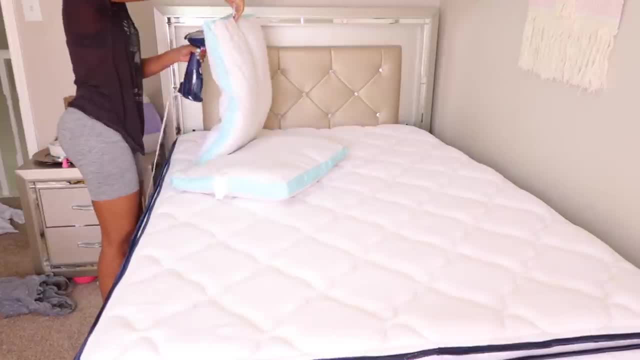 Be careful with it, because I did burn myself a couple of times. I'm just using my hand steamer. It's for garments, but I'm using that to steam the pillows and the mattress. You may have seen me do mine if you have already watched my deep cleaning video. 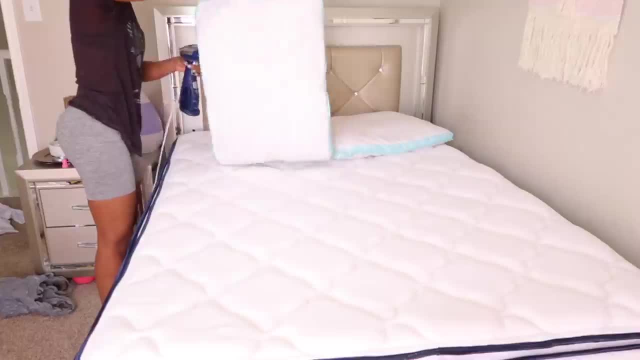 For my master bedroom. if not, check it out, it'll be linked down below. But I don't like to put my pillows in the washing machine because I have an agitator and it just destroys the pillows, So I steam clean them. I'm also going to steam clean the mattress because I try not to put. 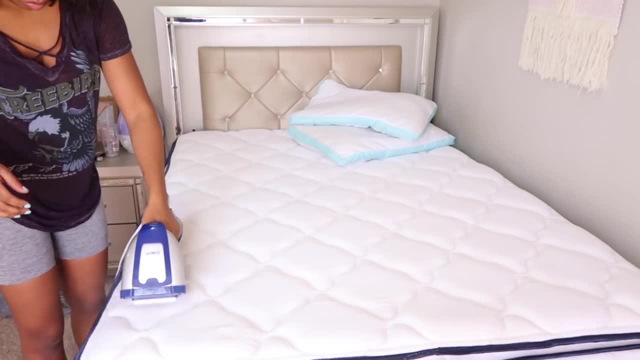 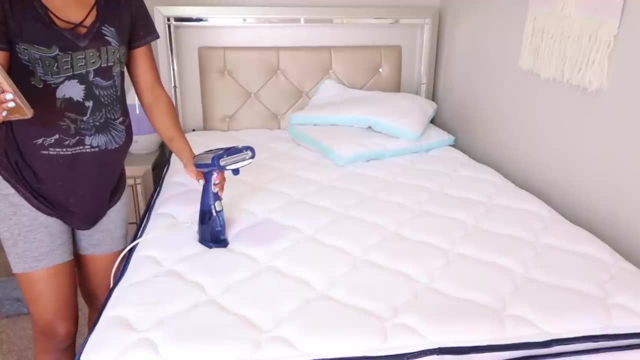 anything really wet on the mattress. It may dry on top, but sometimes that moisture gets stuck in between the mattress and mold grows. So I'm just trying to prevent that. So that's about it. Time to book a room, And I'm going to change my clothes because I've got a lot of stuff to do. 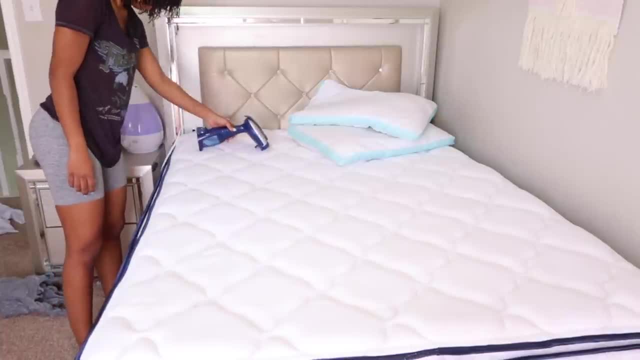 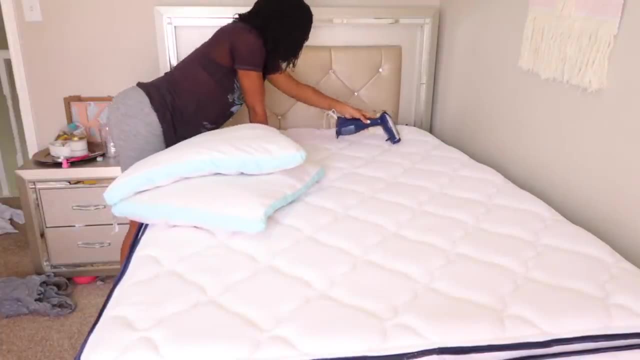 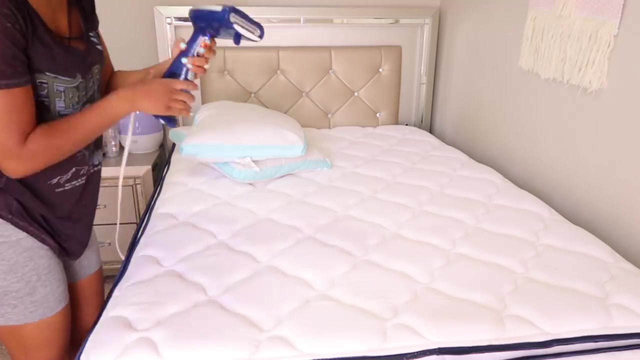 So I'm going to get ready and start making breakfast. This is my breakfast. I've got a lot of groceries And this is the lunch box. I really like to make breakfast right now, So that's what I do. Breakfast is going to be really good. 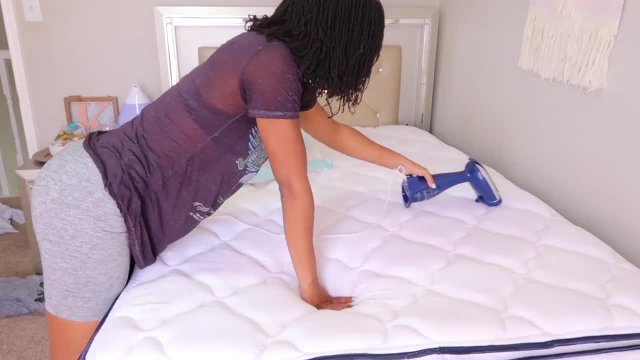 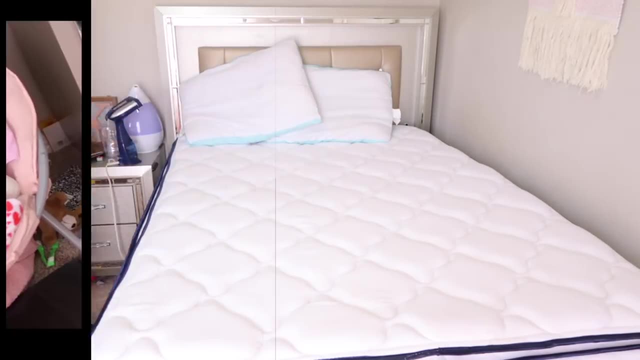 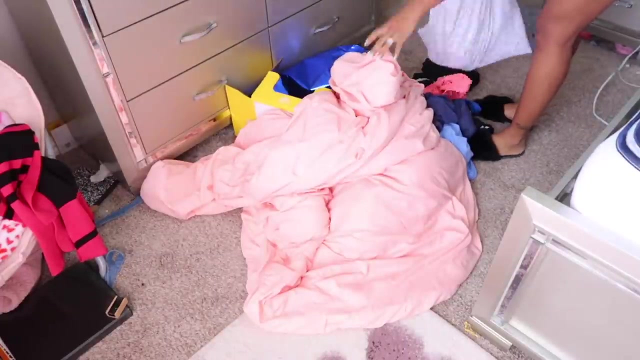 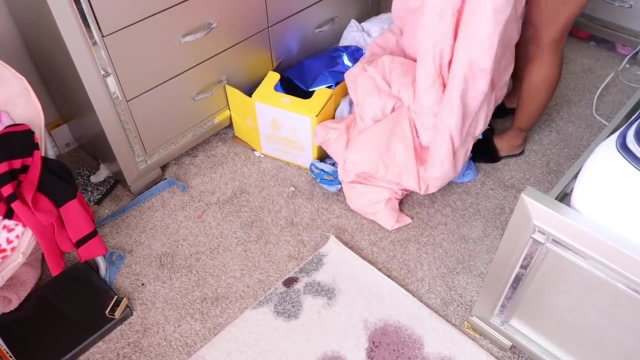 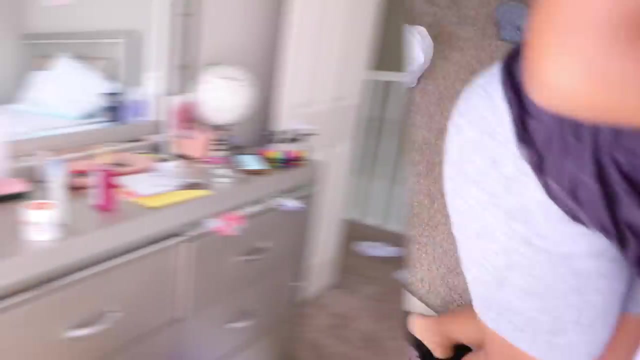 if you're new here and this is your first time watching one of my videos, welcome and thank you for clicking on my video. my name is Karima. I'm a married, full-time working mom. I got two kids. I'm a registered nurse and I pretty much do YouTube full-time as well. I love making cleaning. 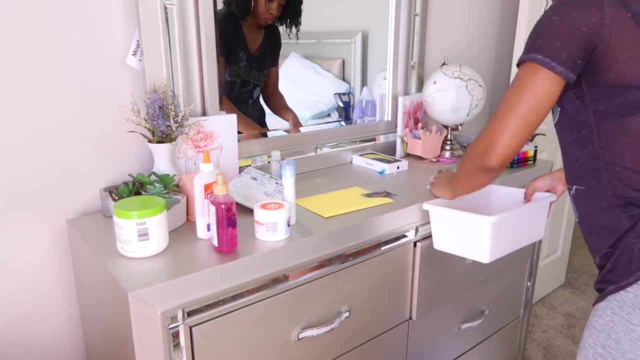 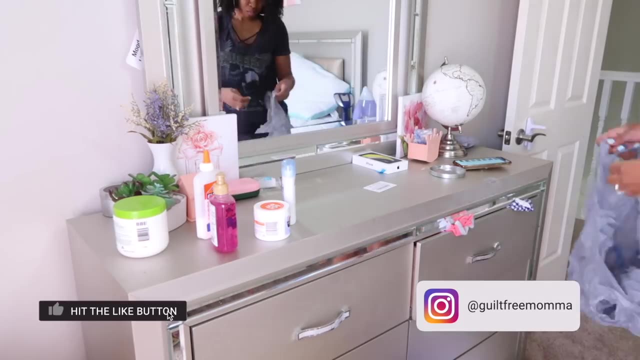 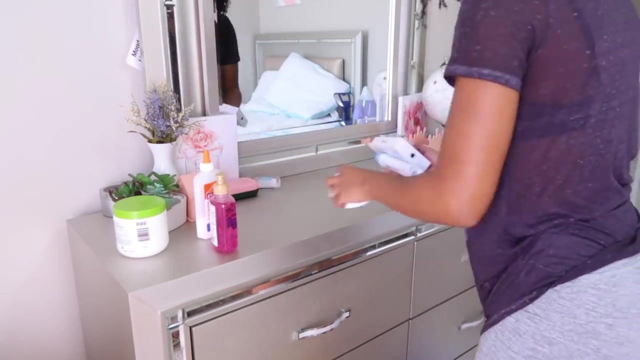 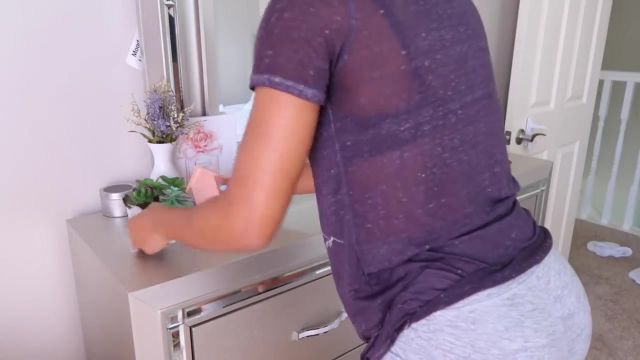 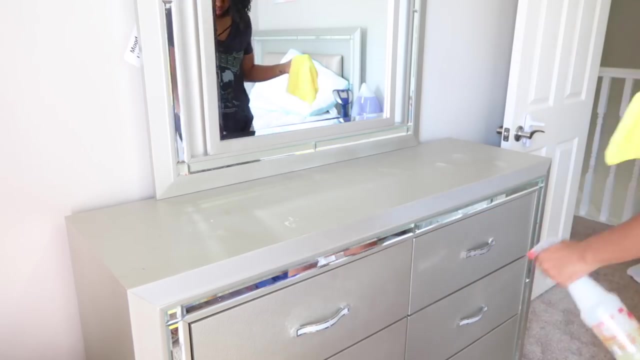 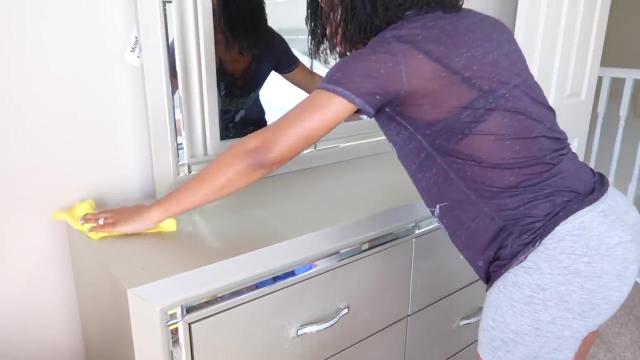 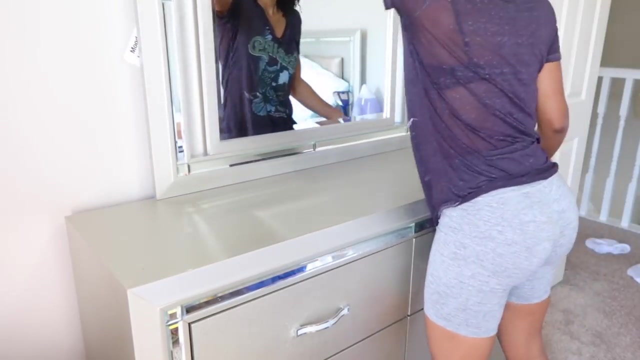 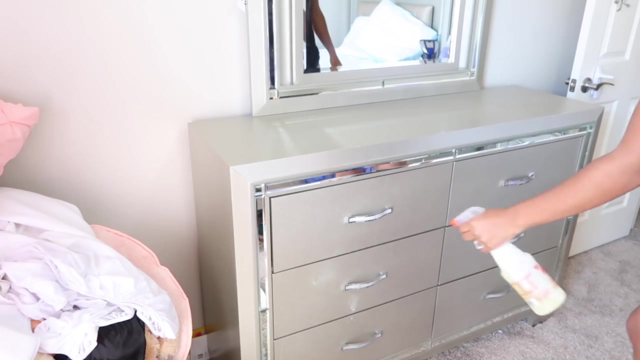 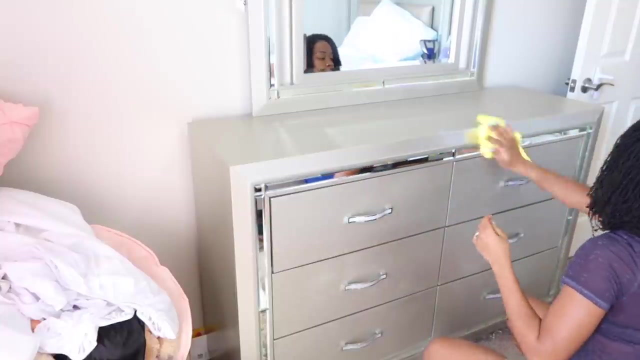 motivation videos and kind of just hanging out with you guys. I love this community, so if you enjoy videos like this, please consider subscribing up the phone. if you tell me I'm gonna meet you alone, if your um brush其实 dancing you on my me on your lips, so sweet, both understanding. when we're a team, nothing can get to me. i'm yours for. 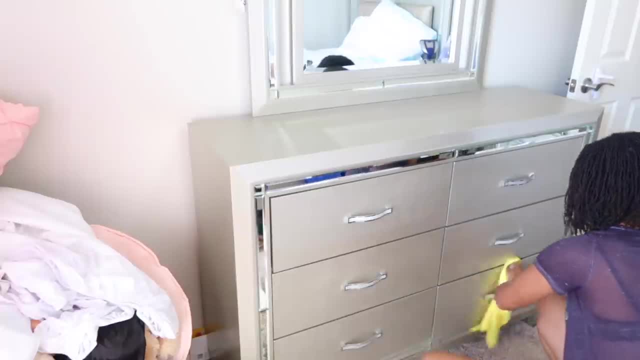 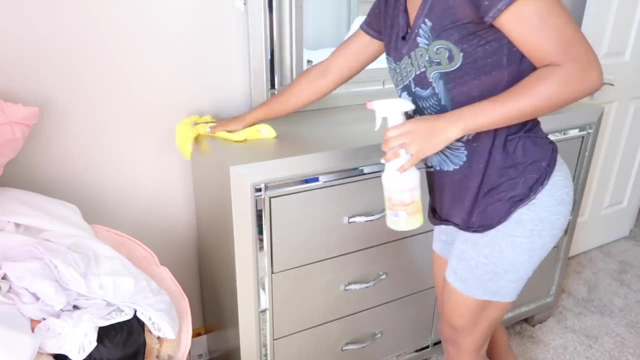 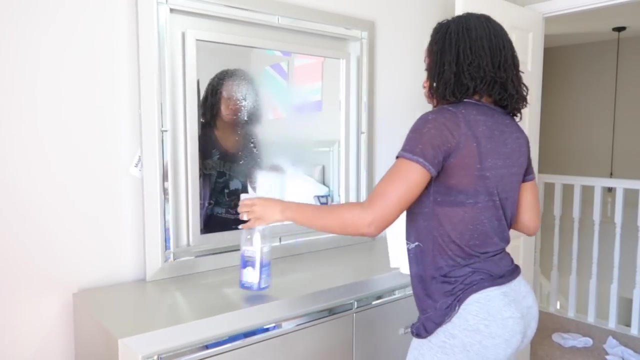 the ticket, every part, all of my art you get. i don't fear nothing when i'm with you and, baby, when you're with me. you call me every night, call me every day. i just wanna get you alone now. trust me when i say we gonna be okay. we just gotta boom bada, boom bop. i don't wanna fight. 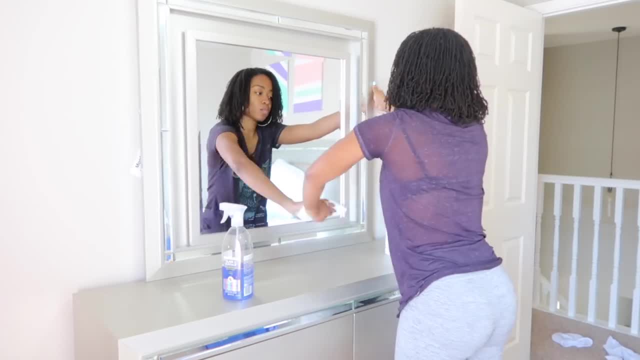 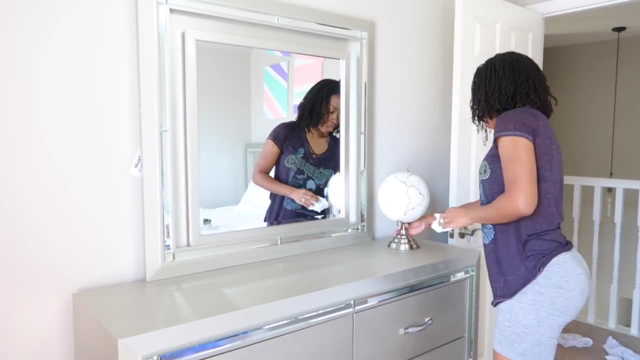 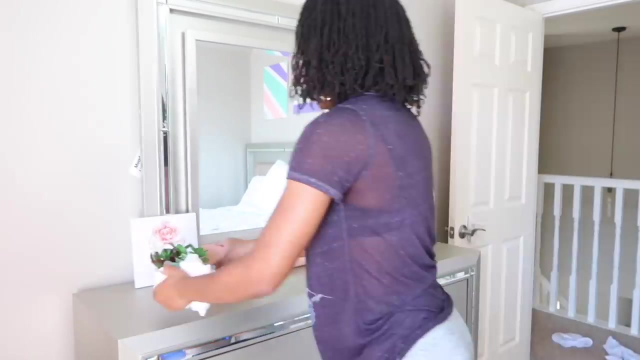 you know that i'm right. baby, let me talk to your body. we gonna be okay. hear me when i say: if you need me, i'm gonna be by your side. if you want me, i'm gonna be there. all right, if you're on me, i'm gonna treat you the right treat. so i just wanted to take a minute and share a snack. 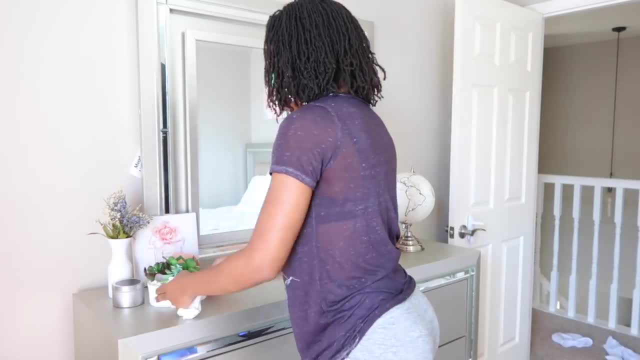 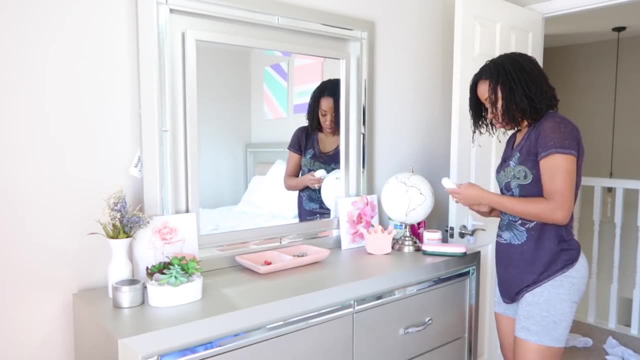 that i've been loving lately- and if you guys are regular viewers then you already know this- but i been loving my built bar protein bars. i will show you guys all the different flavors in a minute, but it is just something that has really been curbing my sweet. 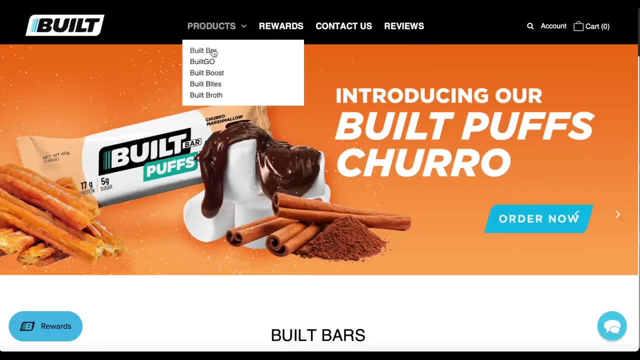 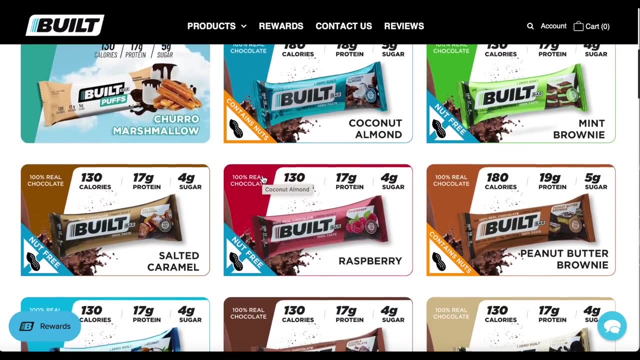 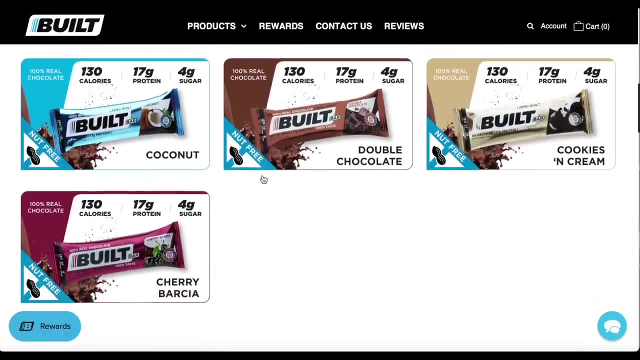 tooth and really just kind of giving me the energy to get through all of this cleaning and just work. it's a nice snack at work. you guys, if you're new here, i'm a registered nurse and i don't get to eat a lot. i don't take a lot of lunch breaks, so it is nice and quick to pull out a protein bar. 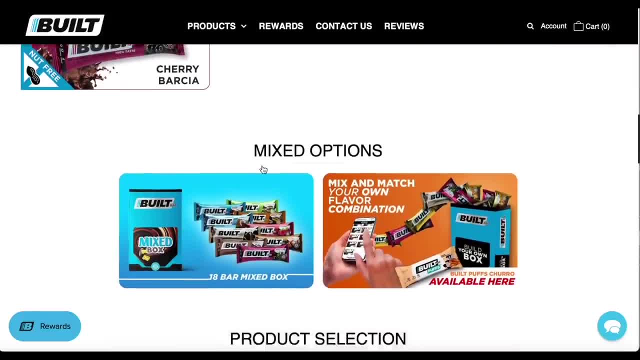 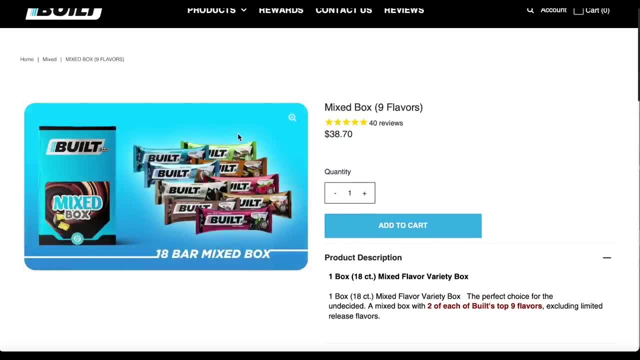 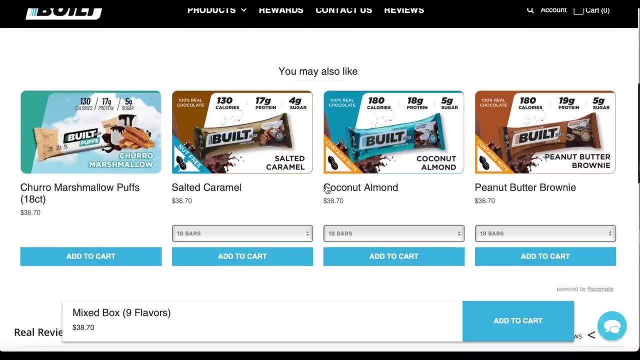 billboard has 18 different flavors to choose from, so i promise there will be something on there for everyone and if not, they have a variety box so you can just test them all out. that's what i did and i found so many favorites. the consistency of the bar is kind of like a candy bar with nougat inside. 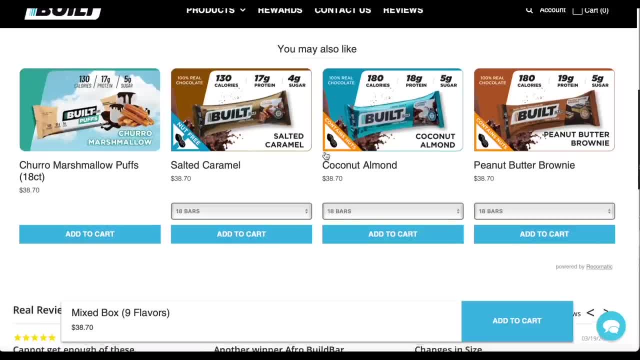 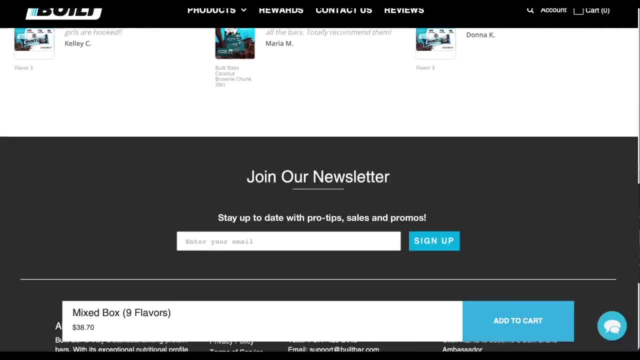 and it actually tastes like a candy bar, so it's more of a treat than a protein bar, but the benefit of it all is that it is low in calories, low in sugar and high in protein. one of my personal favorites is the peanut butter brownie. i love any of the peanut butter brownies that are out there. 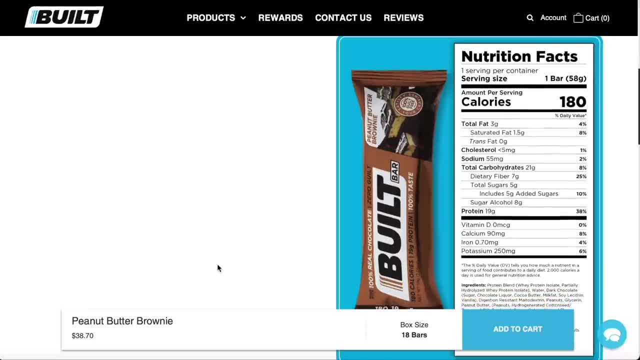 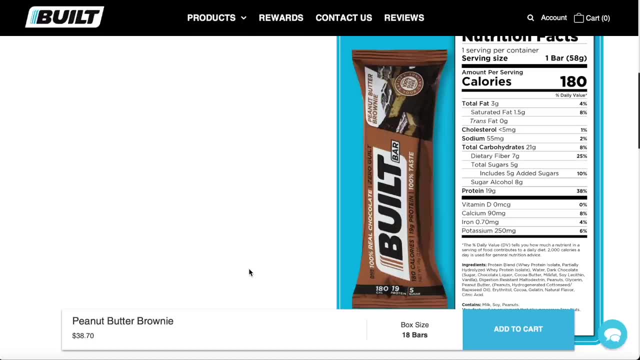 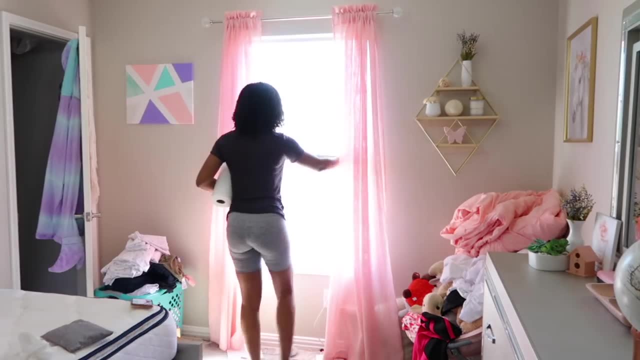 i love anything- peanut butter and chocolate, and the best part about it is that this bar only has 180 calories, 19 grams of protein and only 5 grams of sugar, so it's really a guilt-free treat. if you're into protein bars or you're looking for a healthier version to a candy bar, consider giving. 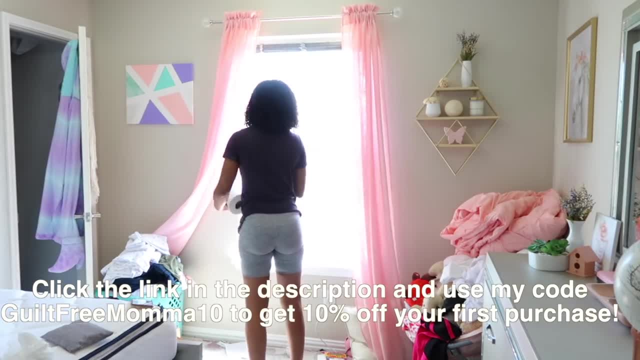 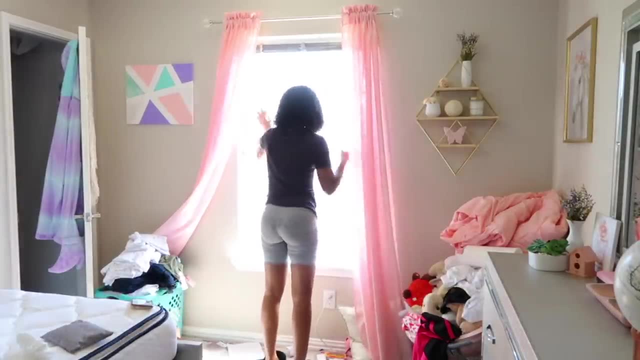 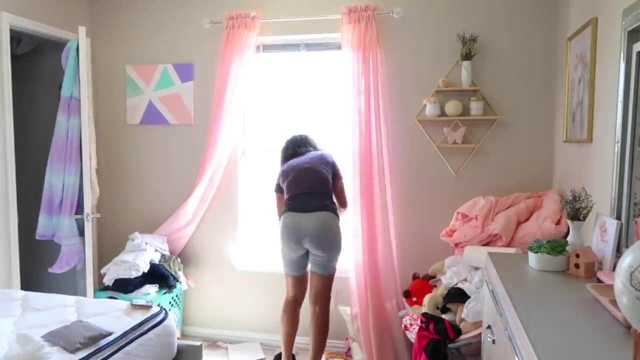 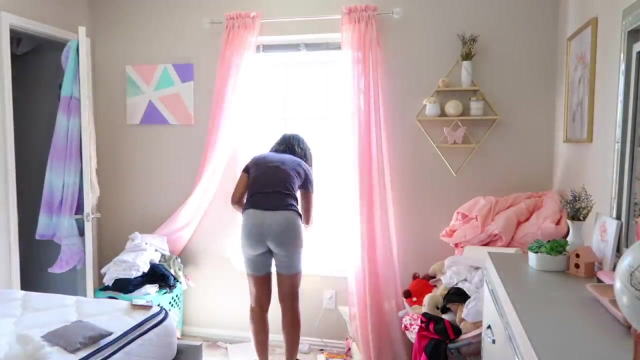 built bar a try. it's really good and if you use my discount code you can save 10 off your order. now back to the cleaning. it's really difficult to clean a window on camera because of the sunlight, but i'm just basically wiping down the windows with my method glass cleaner and i'm just going. 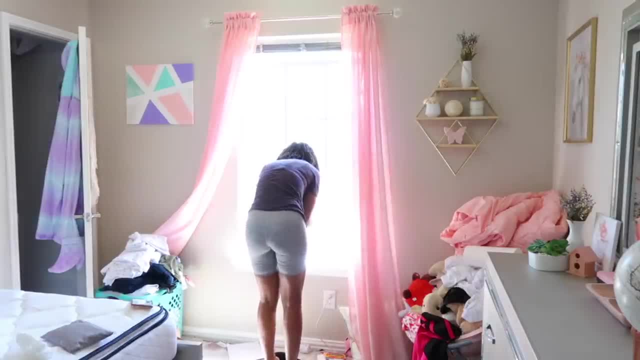 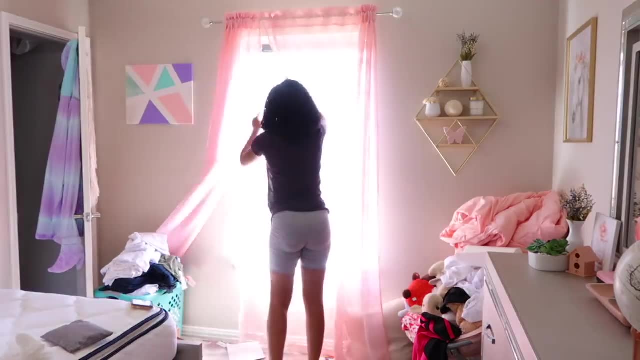 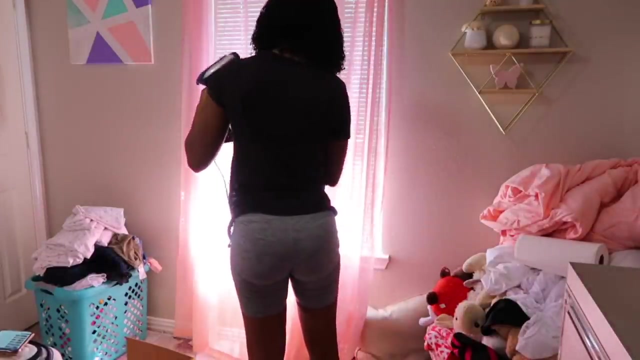 to clean out the window sill. the kids room really wasn't that bad because i have cleaned their window seals before, so i just used a little bit of awesome spray and wiped it down. now i'll be honest here. i wanted to take all the curtains down and wash them like i did my own, but i was feeling super. 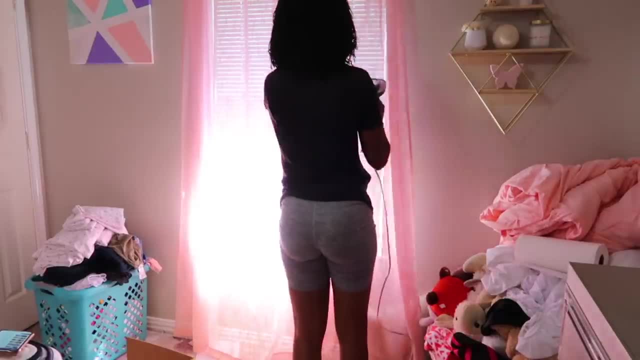 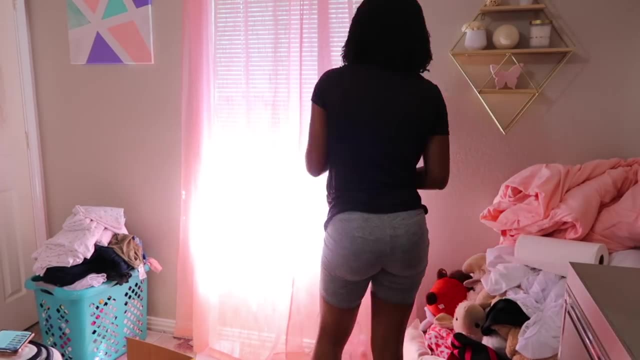 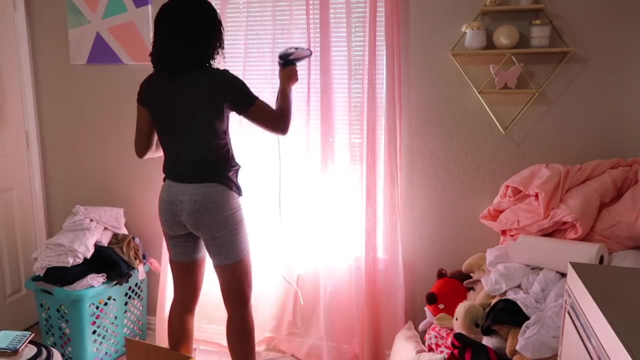 lazy and i just didn't feel like doing that. plus, i wanted to take down kingston's as well and i just wasn't in the mood. so i decided to steam them. at least kill a little bit of germs and get rid of some of the wrinkles at the same time. 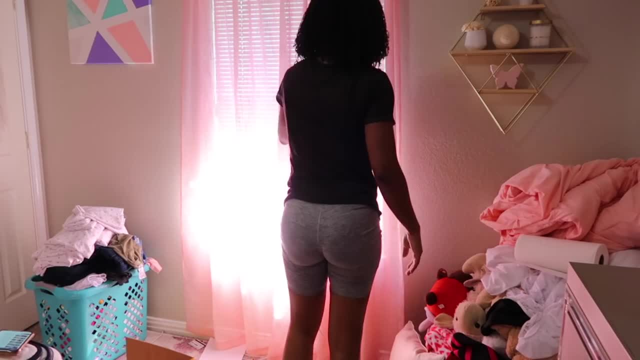 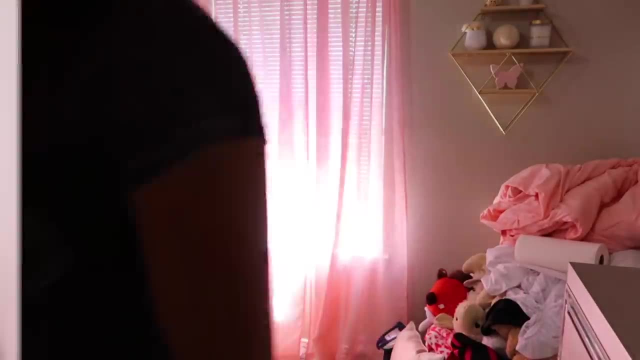 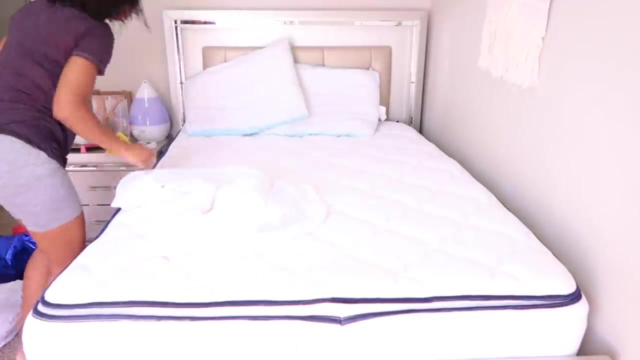 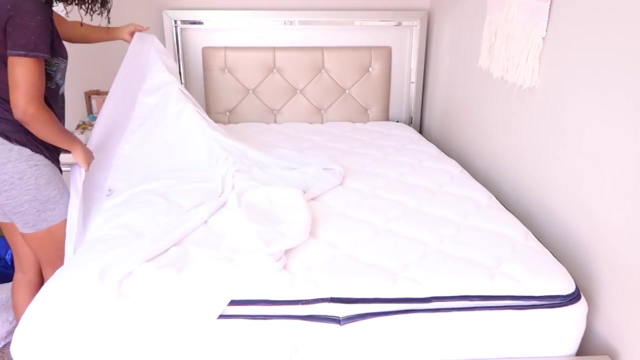 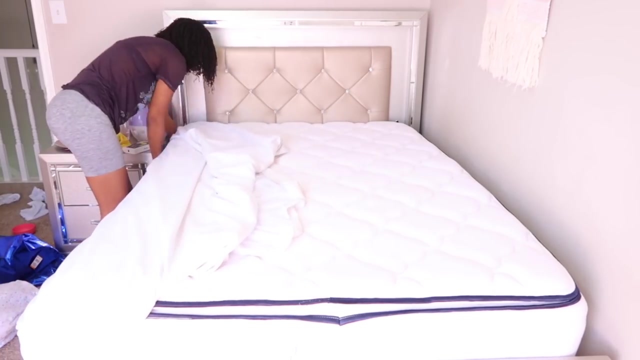 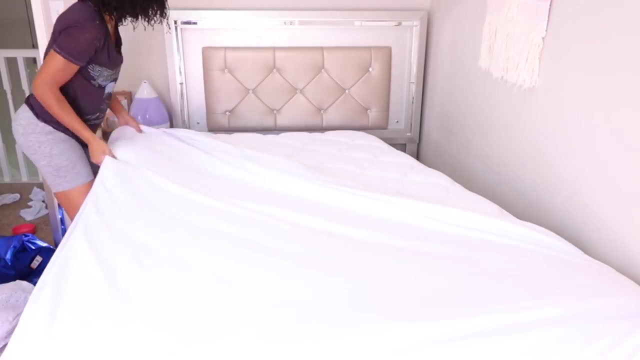 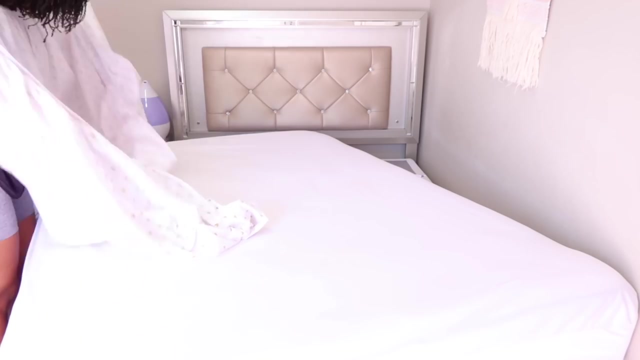 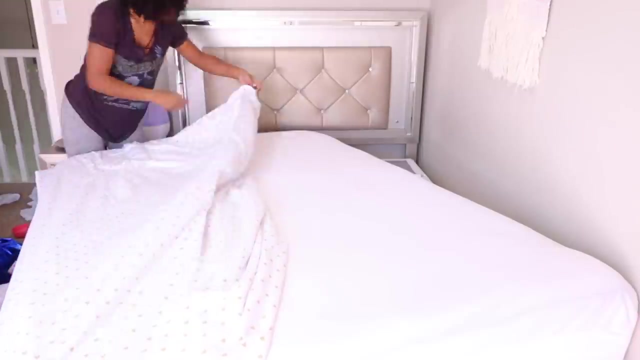 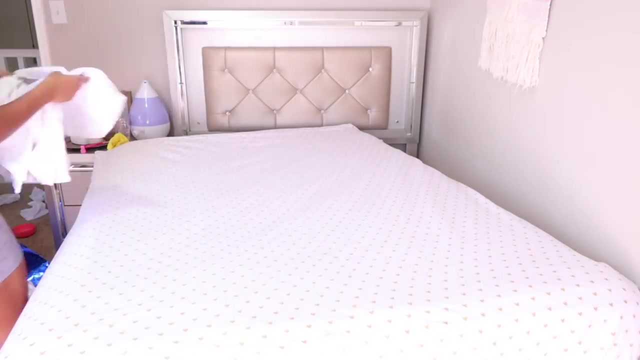 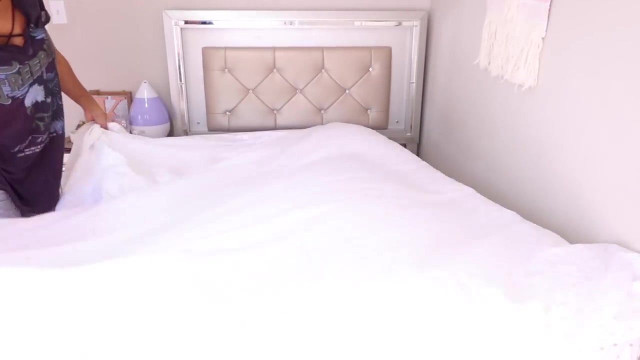 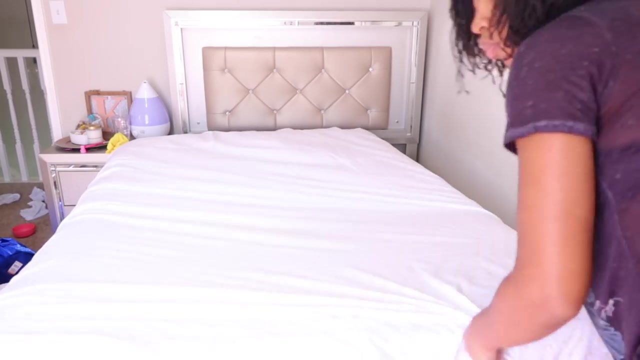 so there's so much more to life than fears is. is it so much more to life than tears is? home is More to life than fears. All I want is a night off. All I need is a night off. All I want is a night off. Take it away, take it away, take it away. 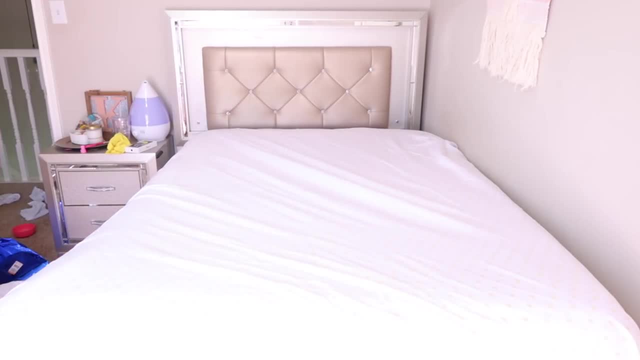 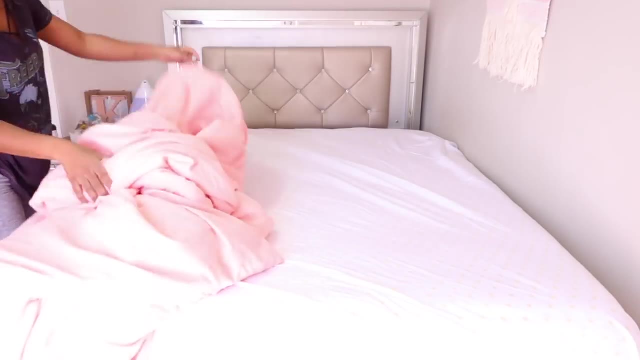 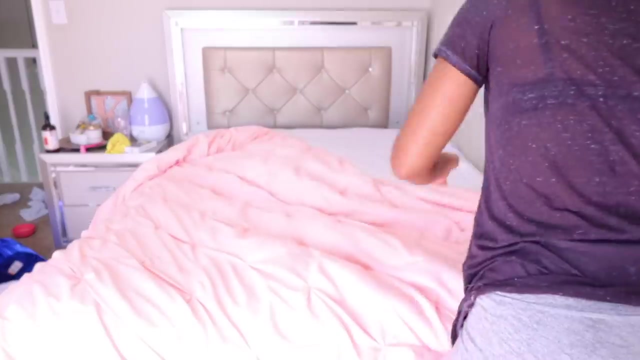 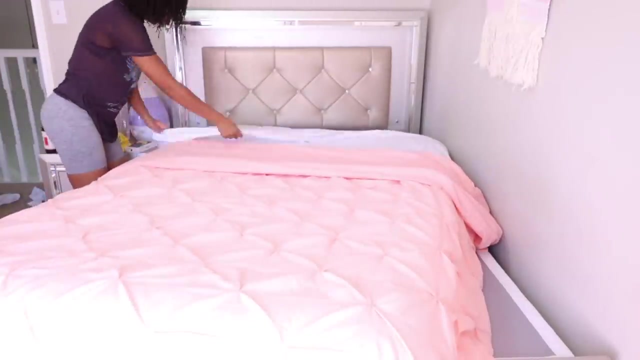 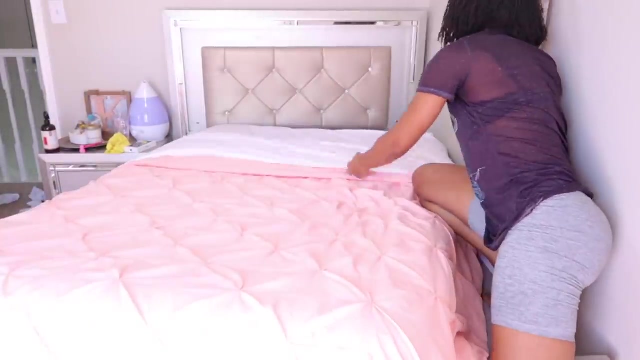 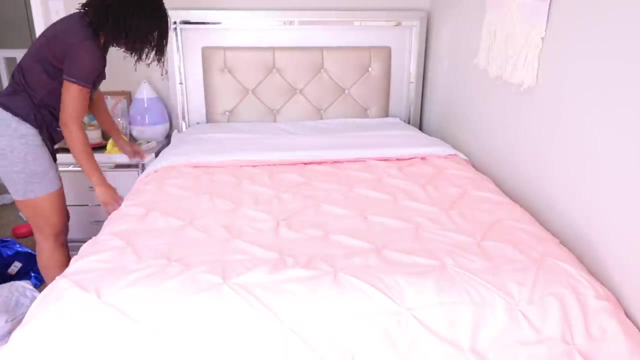 Do it my way, do it my way, do it my way. Free from the pain, free from the pain, free from the pain. A night off, a night off, Baby, I'ma bite for one bite. you said, If you're gonna fight me for my heart. 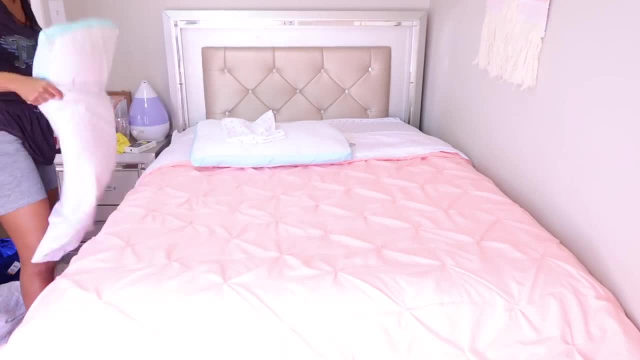 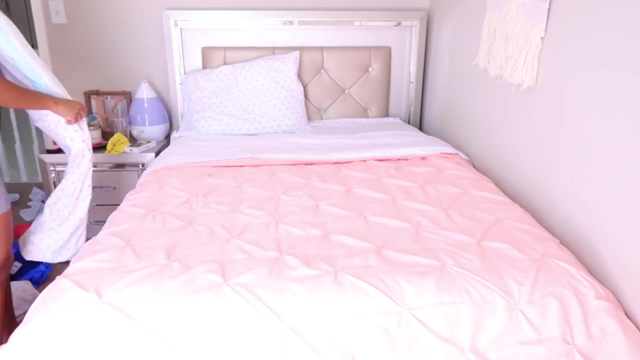 All you're gonna get is blood. oh God, What can I say? I need more than desire, More than just a pretty face. So, girl, you better walk away. Oh yeah, oh yeah. Only one love, if it's harder than fire, Someone who can handle me. 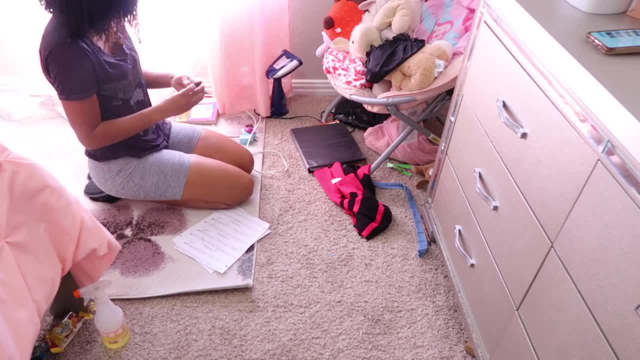 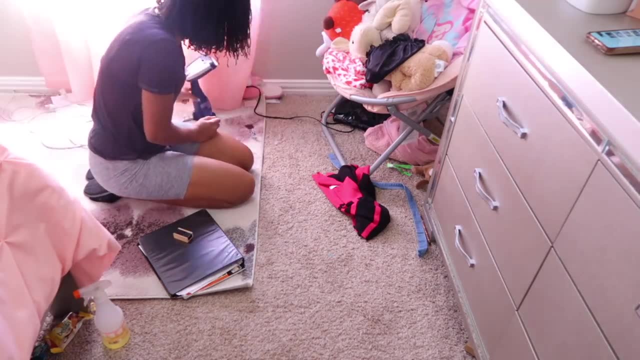 So, like I said before, I really don't go too crazy for her room getting messy. I am just the type of parent that says if your room is messy then just go for it, Just go clean it up. But the one thing I do not like is garbage under her bed and dressers. 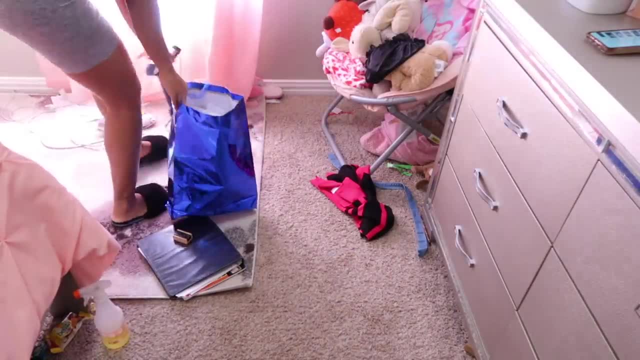 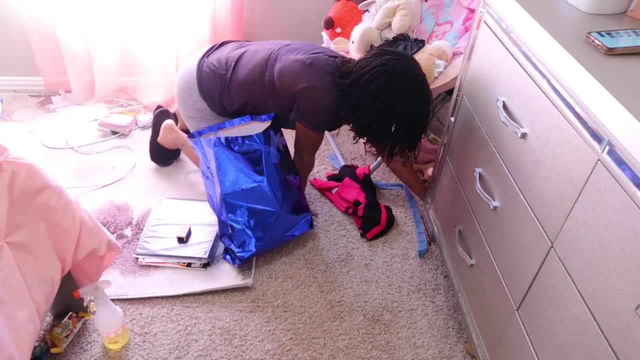 So her dresser is full of junk. I will show you that eventually, Underneath her dresser is full of junk. Her bed I showed you in the beginning of the video. I am not gonna kill myself climbing underneath her bed and pulling things from under her dresser. 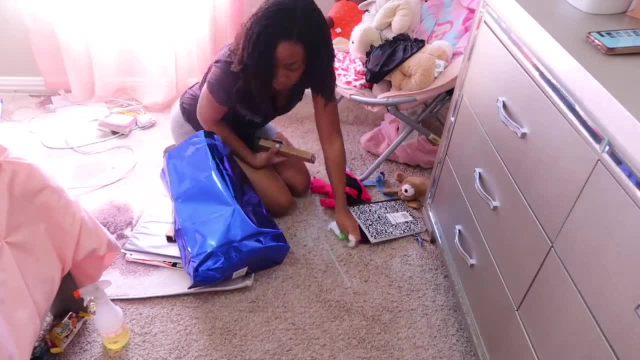 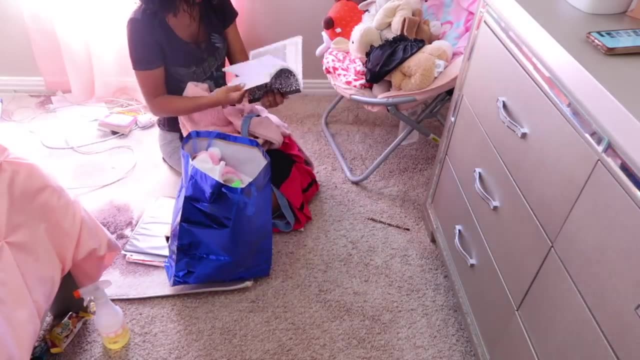 Right, there is when I realized how much stuff she had packed under there, So I left that for her. Her job when she came home from school on this day was to clean underneath that bed, underneath the dresser and the things that was under her night table. 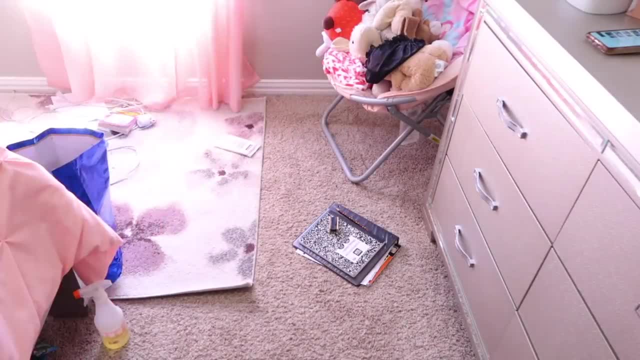 I'm okay with her putting things under her bed, but not trash. I was not happy with the gummy wrappers and cookie wrappers and popped balloons. Things that belong in the garbage should go in the garbage. I'm okay with her storing board games and books. 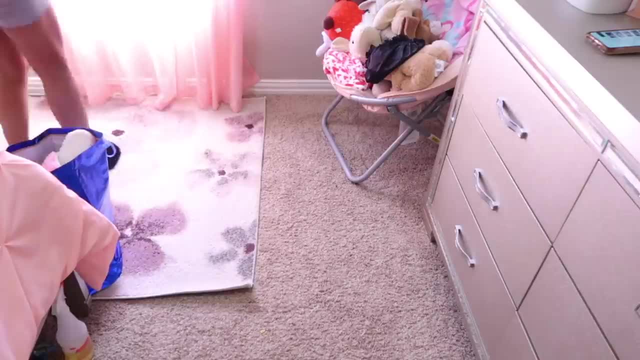 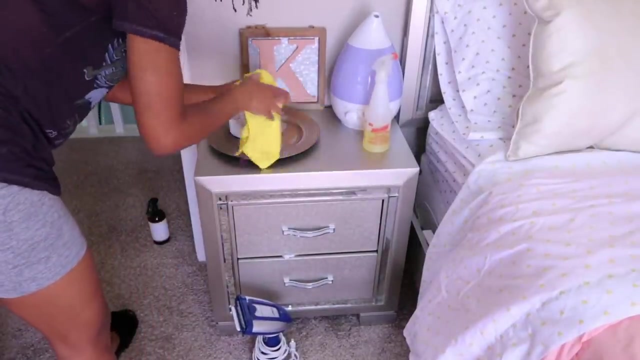 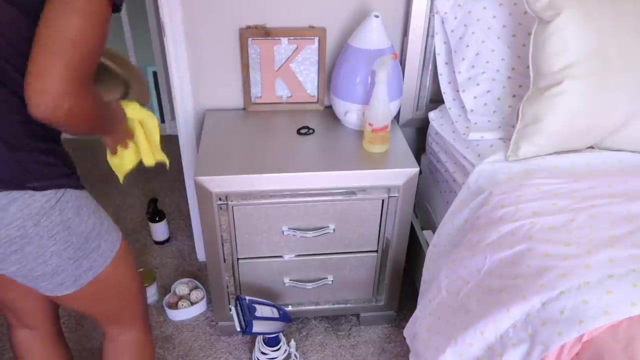 or things like that under her bed, because it is extra storage space, but not trash. I won't leave her. I'm going to start digging down next time. Imagine getting a Принципа. It should make a paper playing game, but a để. 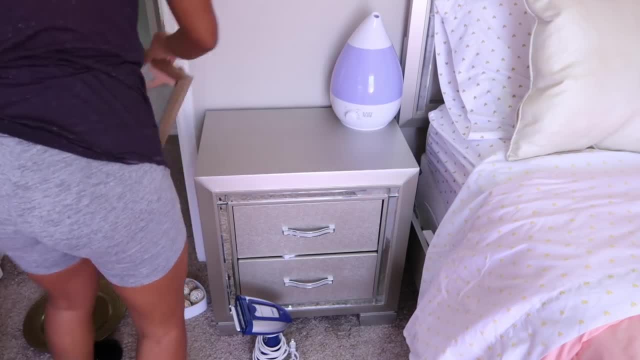 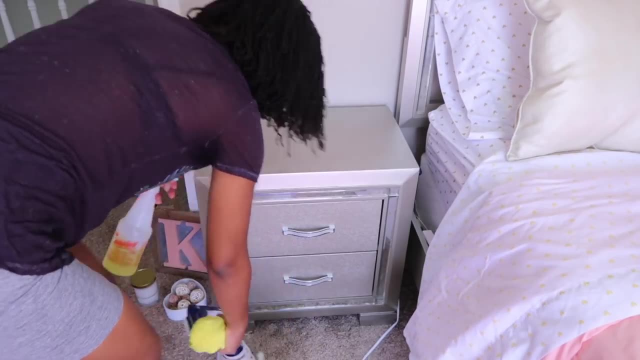 in the more дет Zealand English version is good, but sometimes in the Spanish version also goes extremely badly. You can get it wherever you go, but most of all in overall here. Run away, run away, Baby, I'm a fighter, never backin' down. 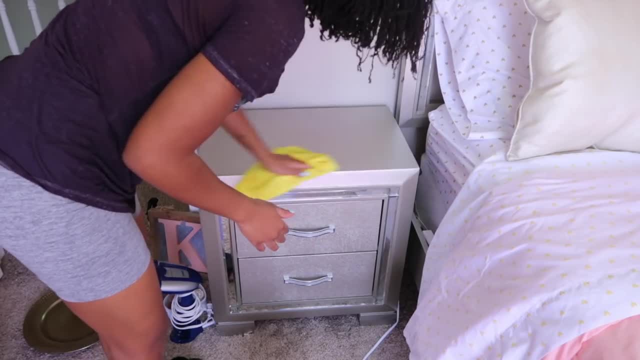 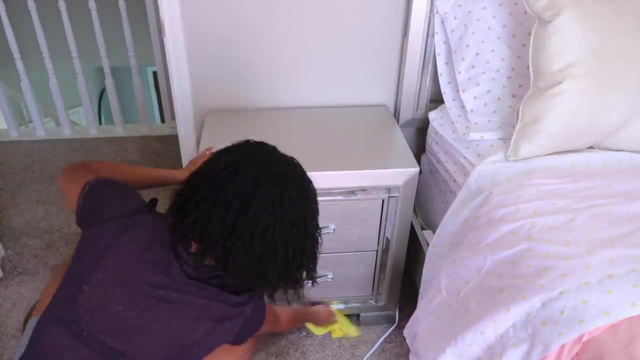 Baby, I'm a soldier standin' my ground. So if you're gonna fight me from my heart, All you're gonna get is battle scars. Baby, I'm a tiger, twenty steps ahead. Baby, I'm a rifle: one bite for dead. 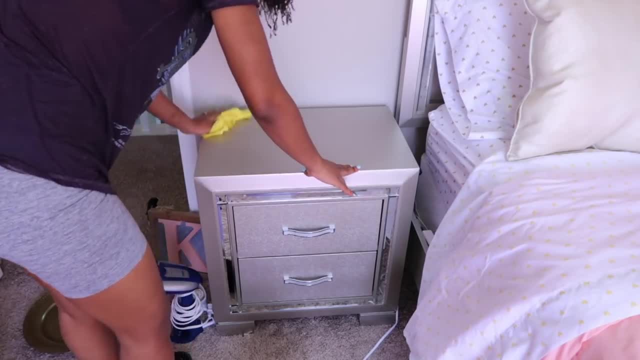 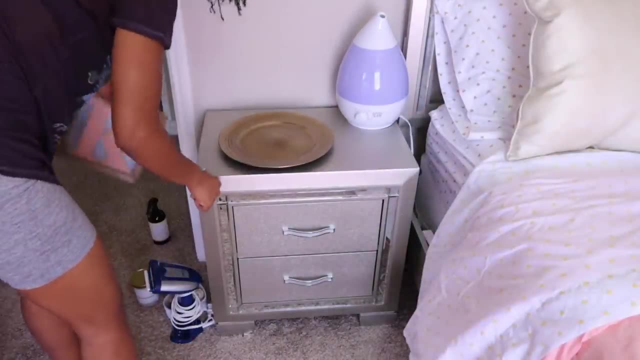 So if you're gonna fight me from my heart, All you're gonna get is battle scars. Baby, I'm a fighter never backin' down. Baby, I'm a soldier standin' my ground. So if you're gonna fight me from my heart, 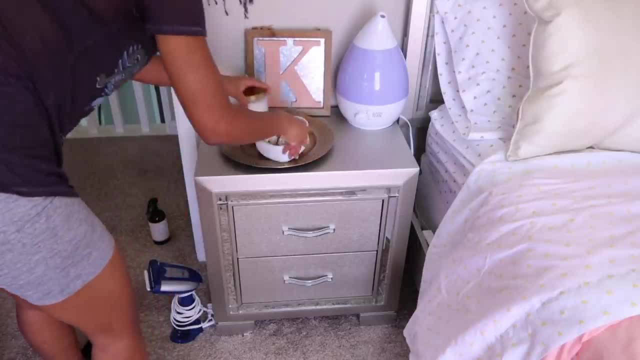 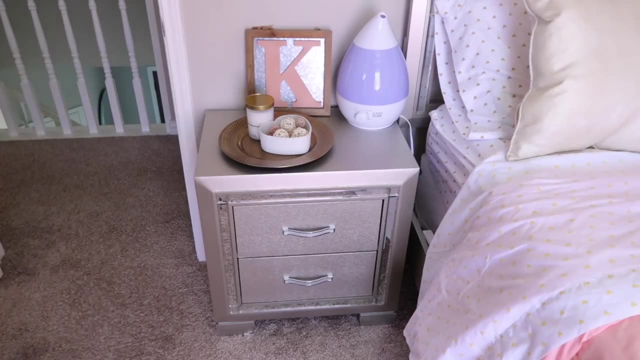 All you're gonna get is battle scars. Baby, I'm a tiger. twenty steps ahead, Baby, I'm a rifle- one bite for dead. So if you're gonna fight me from my heart, All you're gonna get is battle scars. So I did initially plan on shampooing the carpets. 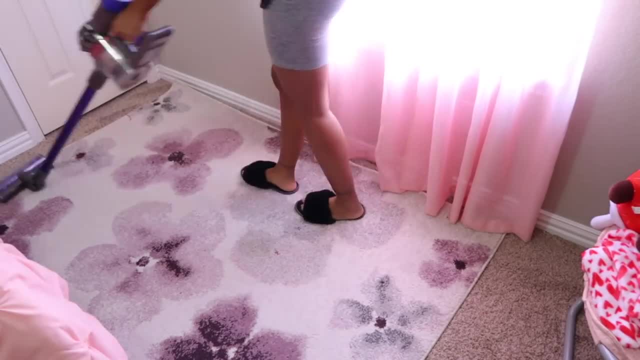 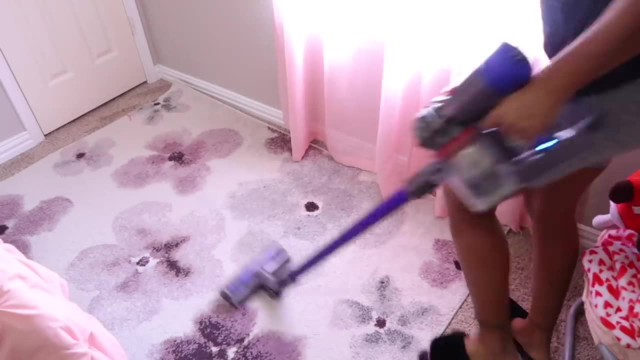 But I realized I don't want to go room by room. I just kind of want to get everyone's room clean So I can shampoo the entire upstairs And not kill myself bringing that thing up and down To go room by room. So I'm just gonna vacuum for now. 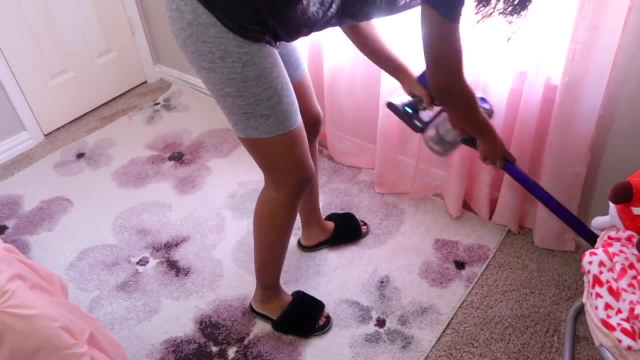 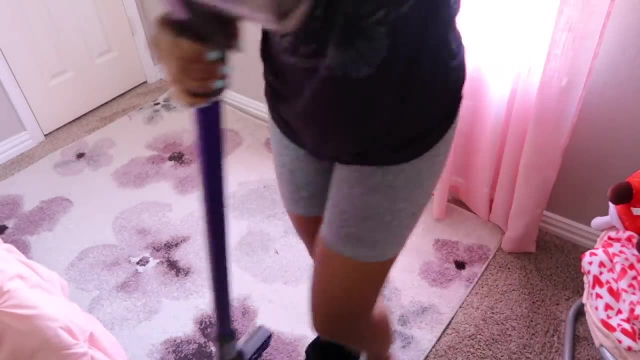 But you will see all the carpets Get shampooed in a future video. But all I hear is noise. I don't have time for Tryin' my luck. I've been too hurt before. You're not that special. Just give it up. I think I've had enough. 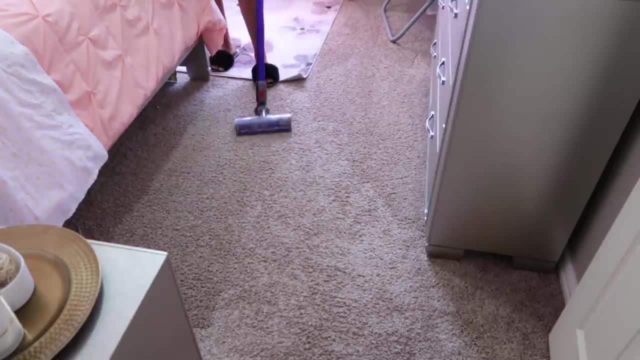 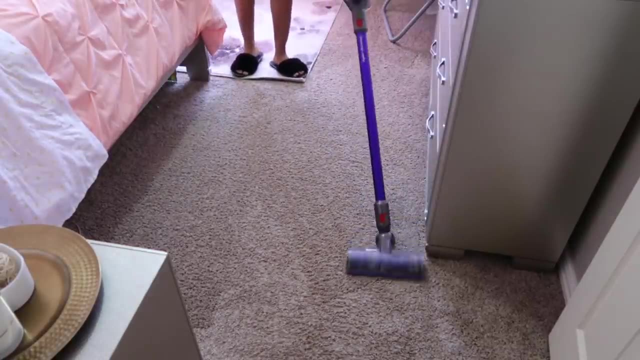 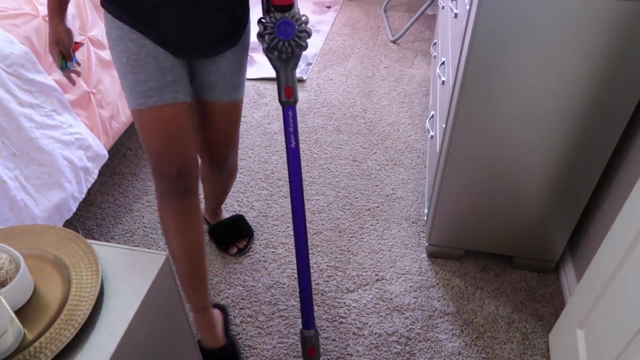 I'm too busy lovin' my friends. I ain't got no love to spare for you. I'ma be that girl to the end. It don't really matter what you do. Guess I have to tell you again Cause you haven't got the news. But you really need to understand. 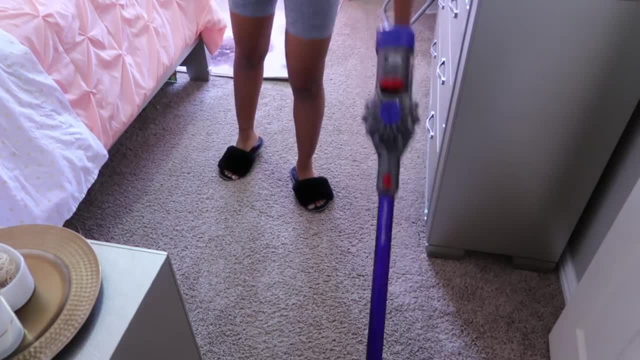 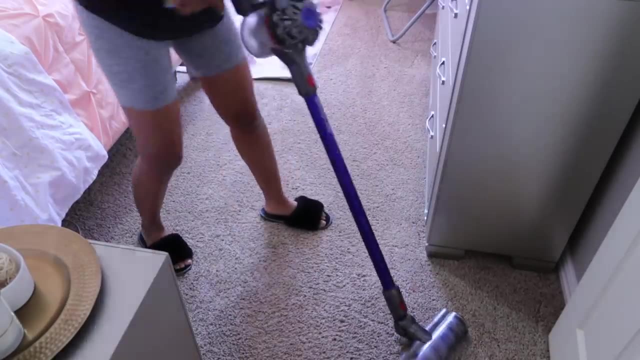 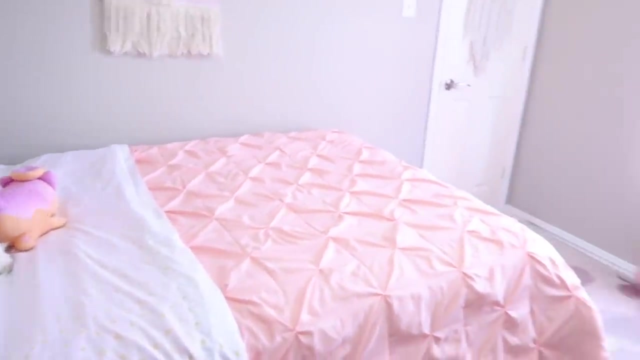 That I don't wanna be your Girlfriend girlfriend. No, I don't wanna be your Girlfriend girlfriend. All I wanna do is tell my Girlfriend's girlfriend So I don't wanna be your Girlfriend's girlfriend. So here is the finished results of her room: Everything kind of in order and nice and clean. 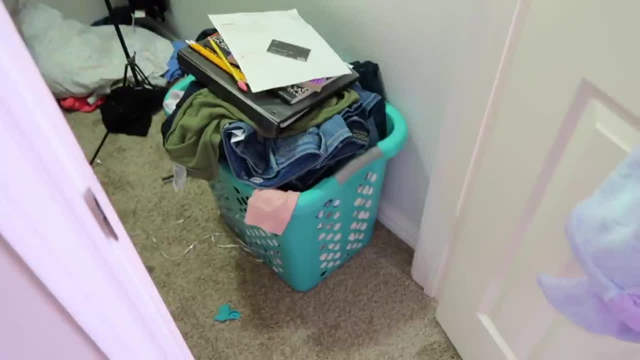 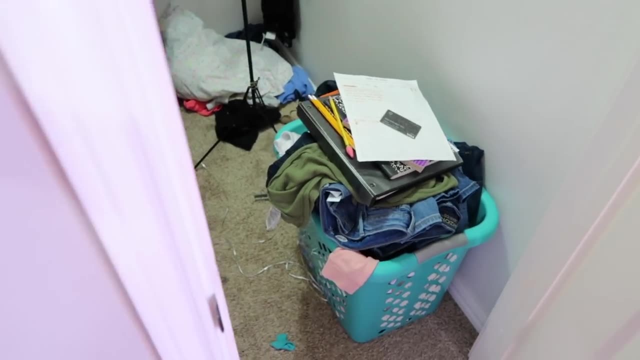 And I will show you guys the few things I did leave out in the video. Leave for her to take care of Her laundry. She needs to put her music book away And fold her laundry. That is all clean laundry in that basket, So she needs to fold it and put it away. 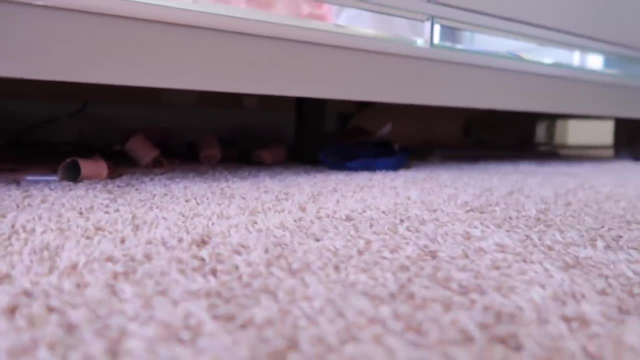 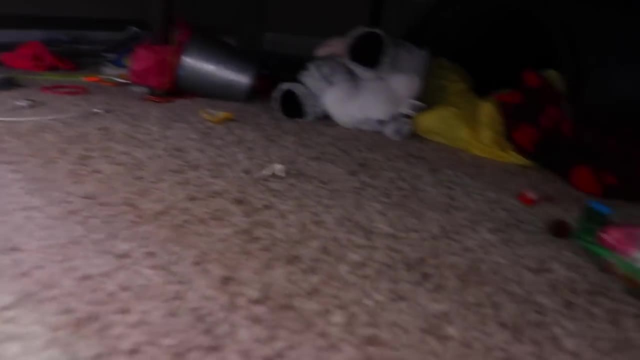 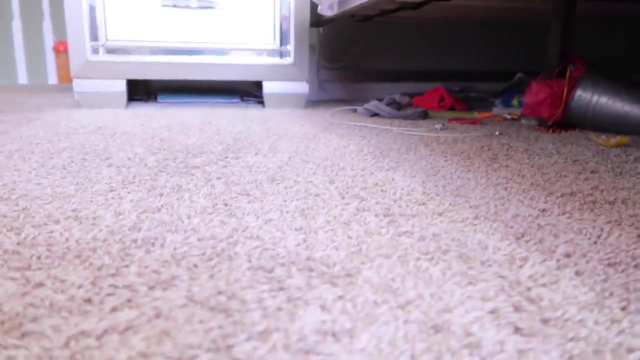 She needs to clean up underneath this dresser And clean underneath her bed And night table. I ain't got no love to spare for you. I'ma be that girl to the end, It don't really matter what you do. Guess I have to tell you again, Cause you haven't got the news. 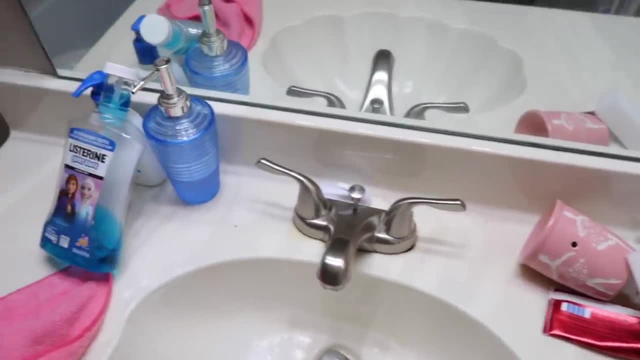 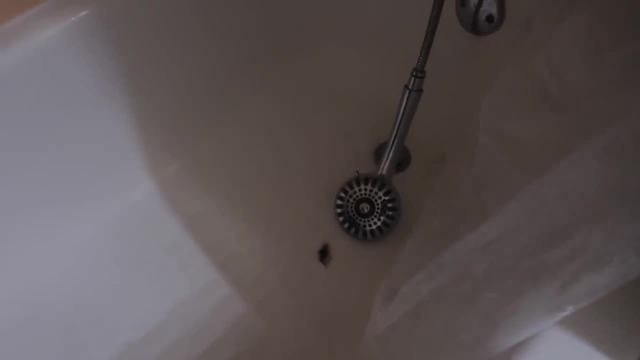 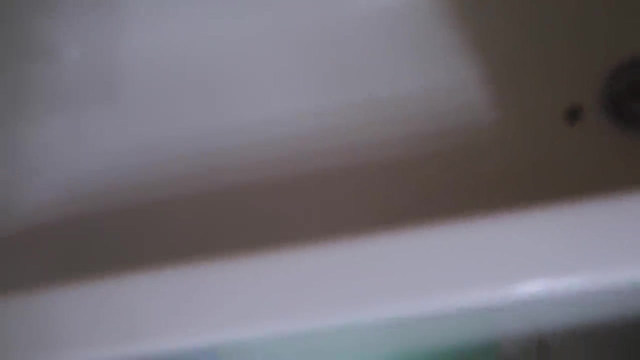 But you really need to understand That I don't wanna be your Girlfriend, girlfriend, So moving right along. I am in the kids bathroom and it is gross. The tub really needs to be cleaned out. That is hair in the tub from Washing Chloe's hair. Why it's still there, I don't know. 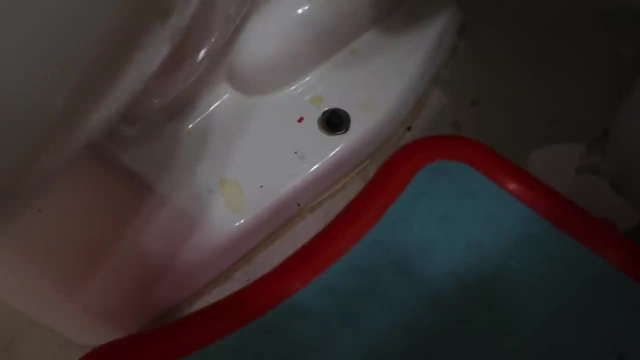 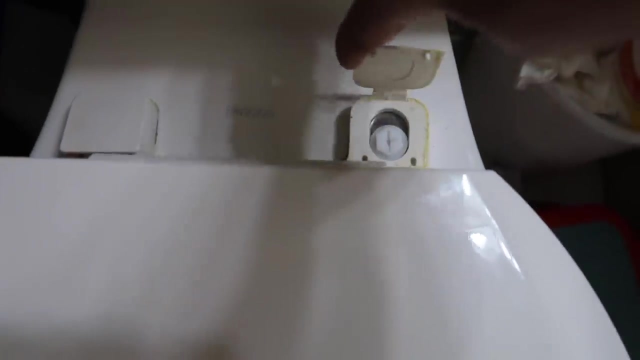 And shout out to all my boy moms. Because it's rough, There's pee everywhere: On the bottom of the toilet, the floor, And the kids do wipe off the back of the toilet But not under the screw holes, So that is full of pee. From my lovely Kingston. 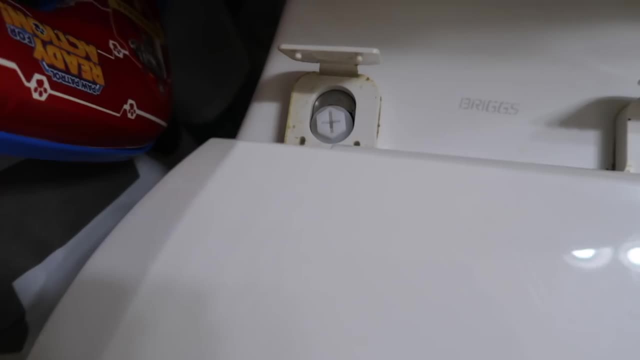 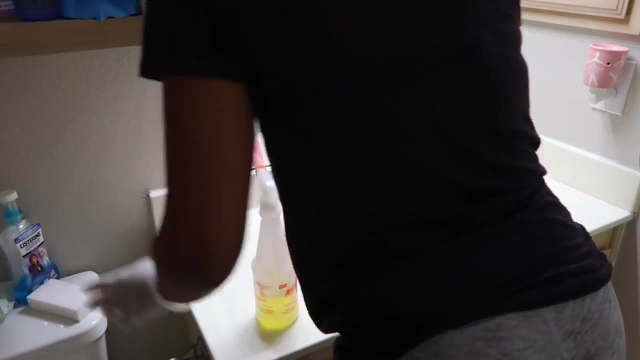 So I'm going to take care of all of that. So I don't wanna be your Girlfriend, girlfriend. No, no, no, no, no, no, no. I don't really have time for you, boy. I don't wanna hear anything more. 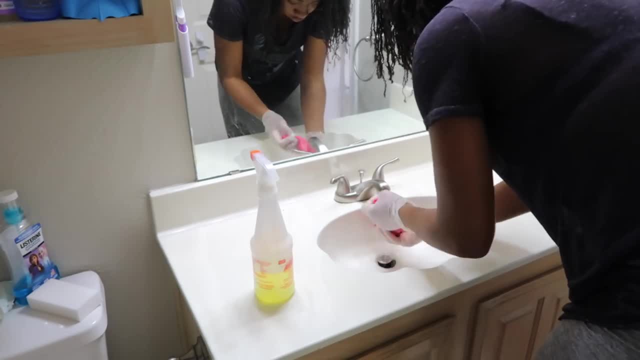 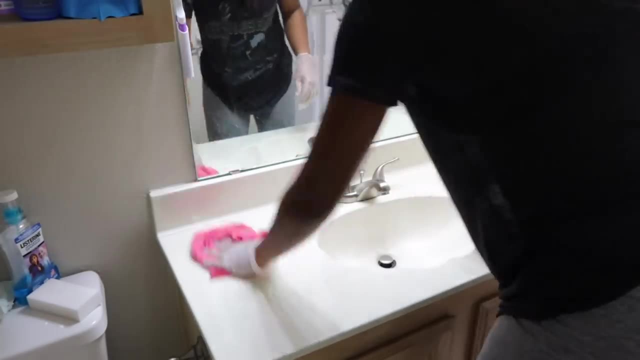 Boy, you really need to understand That I'm not your girlfriend. I just wanna be up in the club, But my girls, yeah, sippin' hot. But my girls, yeah, sippin' hot. But my girls, yeah, sippin' hot. 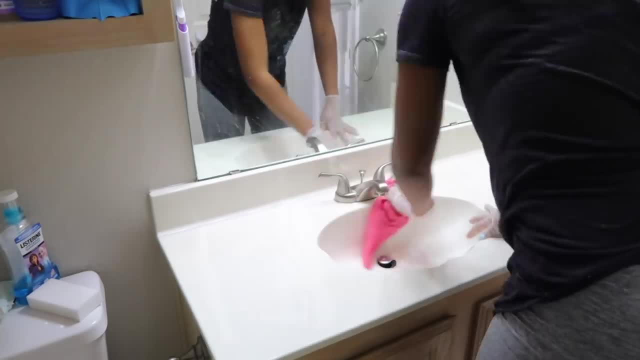 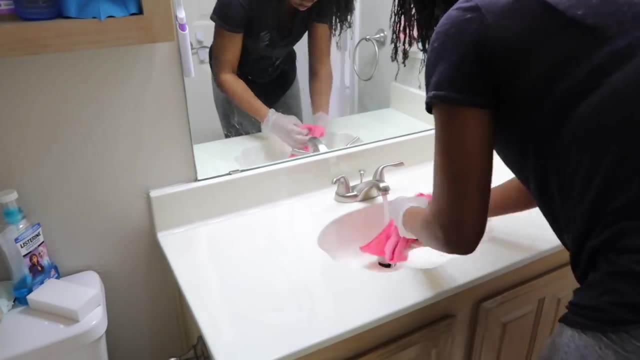 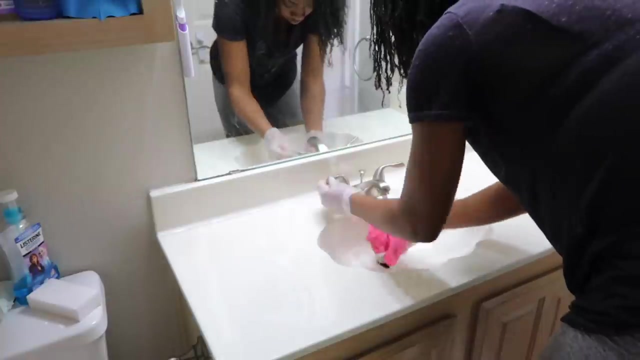 Get a nap up, Never worry about it. love, love, love, love, Cause I'm not your girlfriend. Yeah, yeah, And I never wanna be your Girlfriend girlfriend. No, I don't wanna be your Girlfriend girlfriend. I love when it's time with my 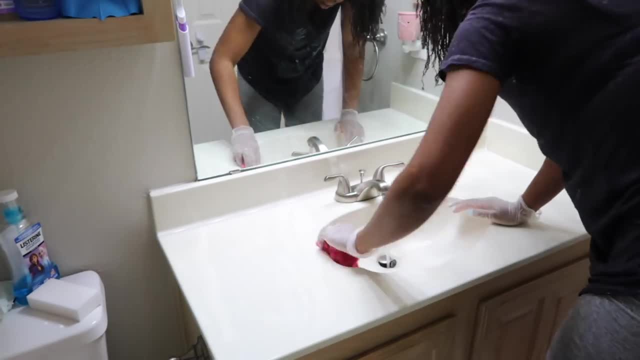 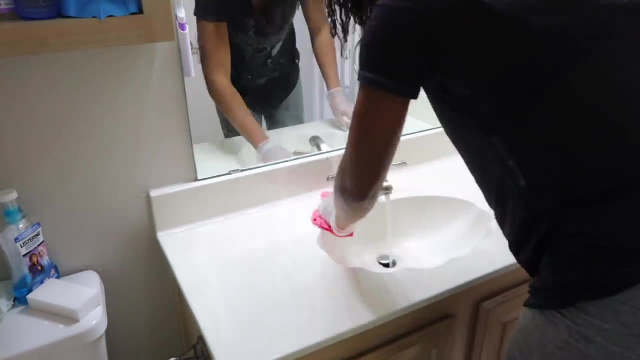 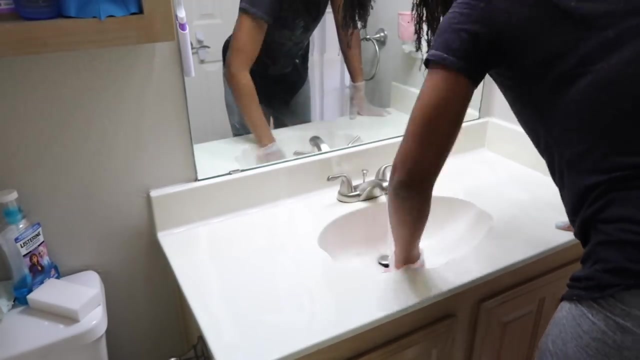 Girlfriends, girlfriends. So I don't wanna be your Girlfriend girlfriend. No, no, no, no, no, no Girlfriend girlfriend. No, no, no, no, no, no Girlfriend girlfriend. No, no, no, no, no, no. 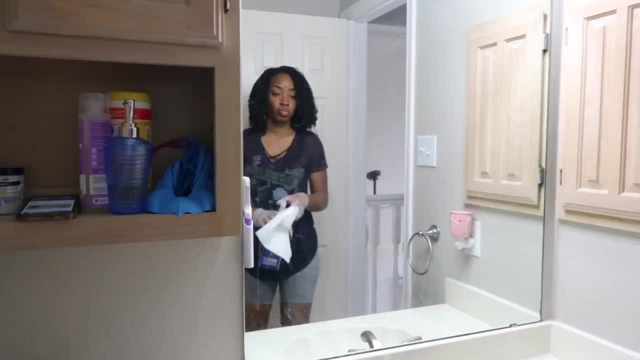 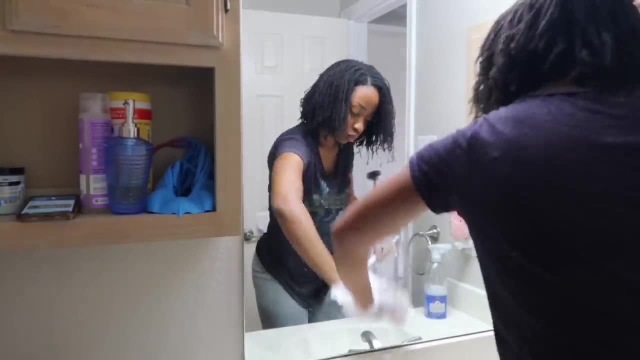 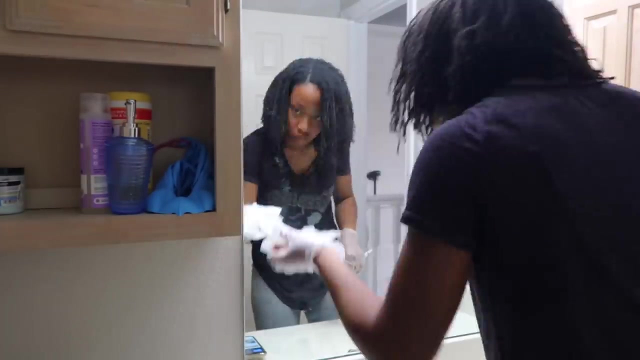 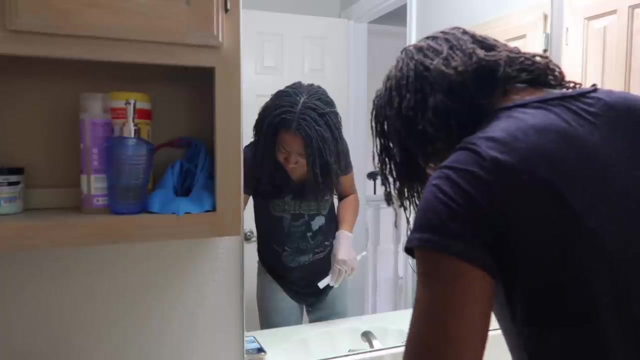 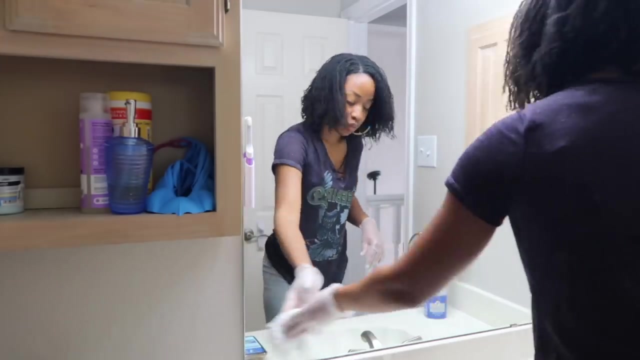 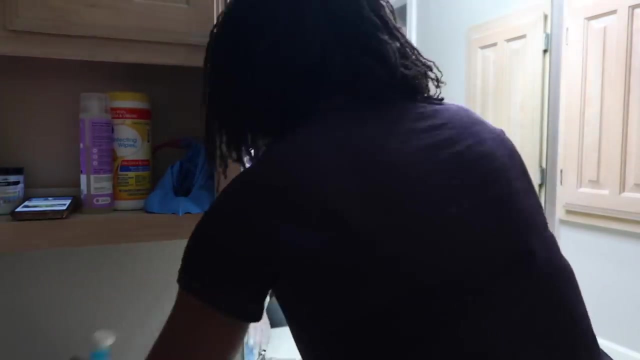 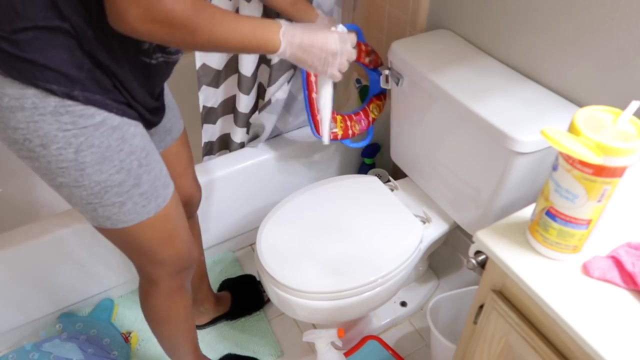 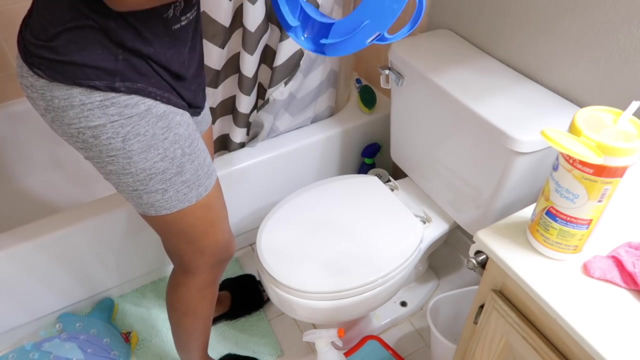 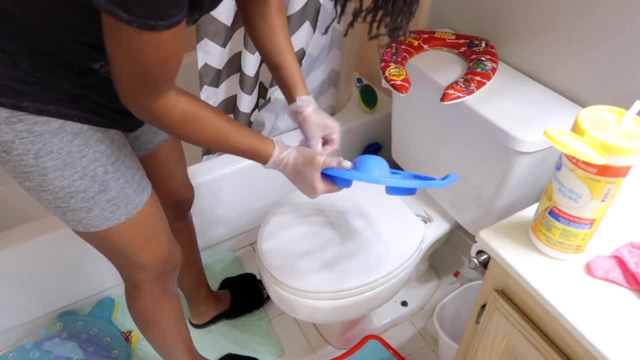 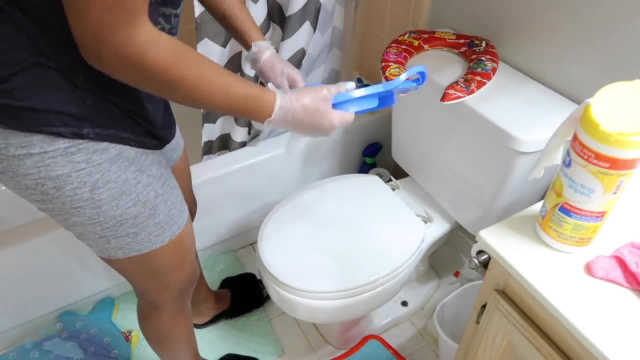 I think I'm off drunk And it feels like I'm in a dream. And it feels like I'm in a dream. I feel drunk, But I'm not afraid to admit. I used to feel safe Next to you, babe. Now I'm thinking I deserve a hit. Maybe someday We could work it out, But I'm afraid It's too late to try. Baby, I don't dare to love you, And you know the reason why. Don't you know I'm way too weak to swim. Can't you feel the waves come crashing in? Running out of safety nets. Cause every night, every night, I fall down in the middle of the night, Screaming oh my god, Cause your love's too deep, You know your love's too deep. I reach out in the middle of the night, Screaming oh my my. 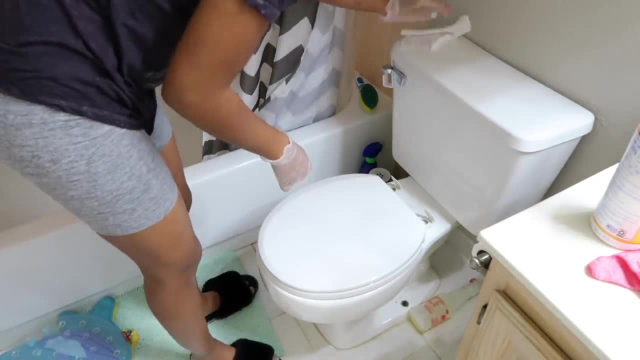 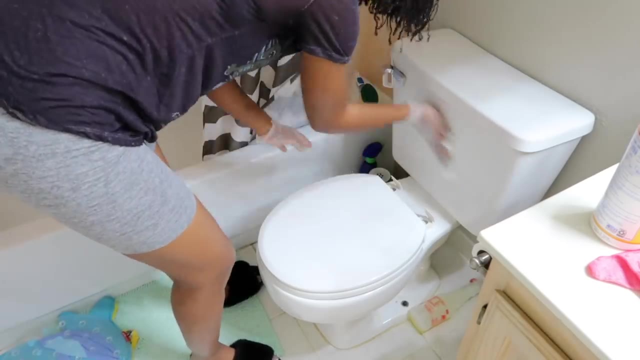 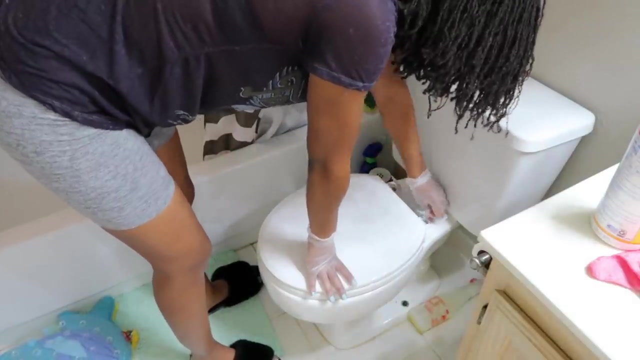 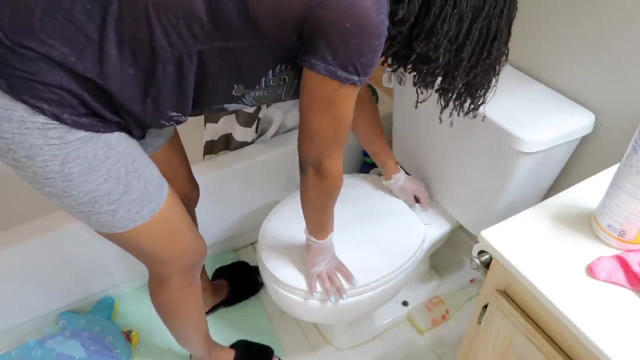 Cause your love's too deep. You know your love's too deep. Love, love, love's too deep. Love, love, love's too deep. Love, love, love's too deep. You know your love's too deep. You know your love's too deep. 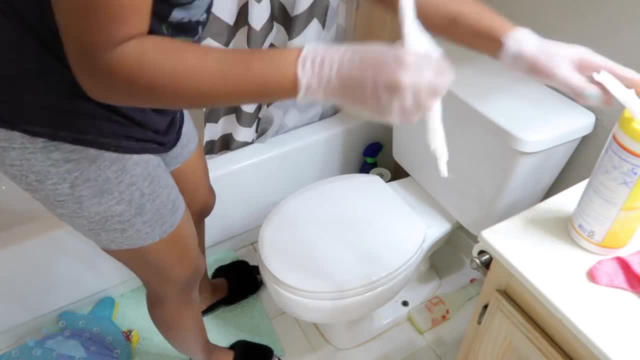 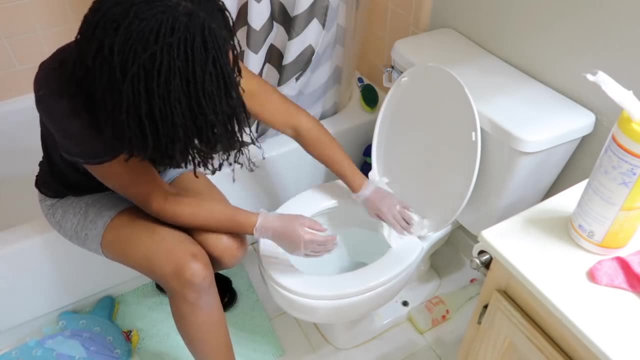 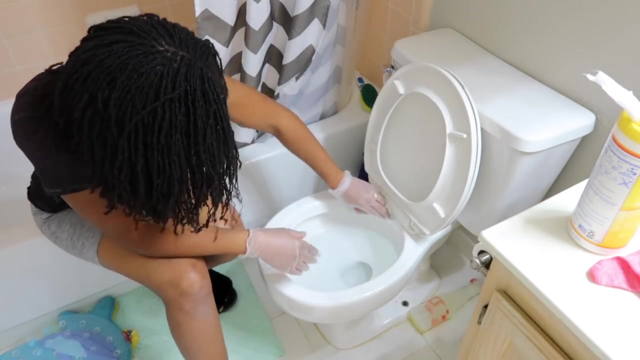 Oh, yeah, yeah, Oh no, no, no, Oh baby, yeah, Don't you know I'm way too weak to swim. Can't you feel the waves come crashing in, Running out of safety nets? Cause every night, every night, I fall down in the middle of the night. Screaming: oh my god, Cause your love's too deep, You know your love's too deep. I reach out in the middle of the night Screaming: oh my god, Cause your love's too deep, You know your love's too deep. Oh yeah, yeah, Work too deep. 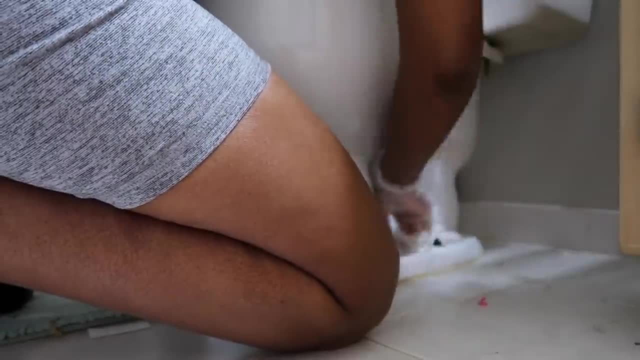 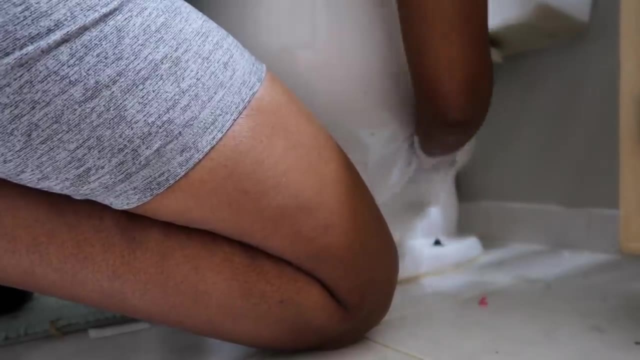 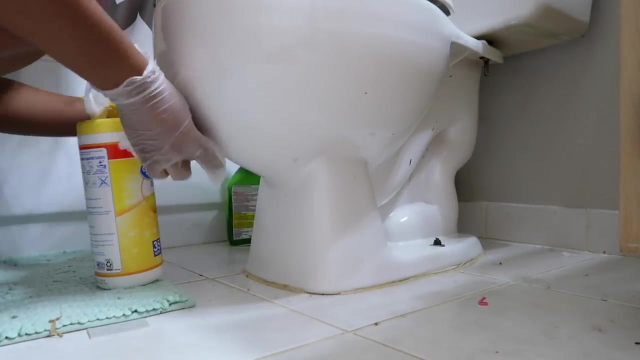 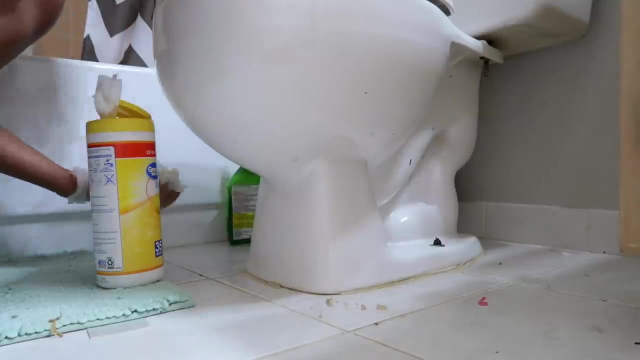 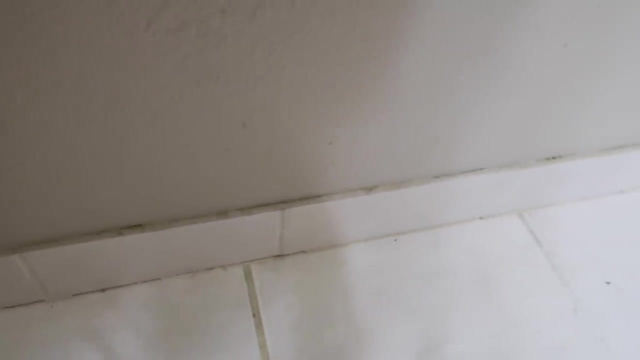 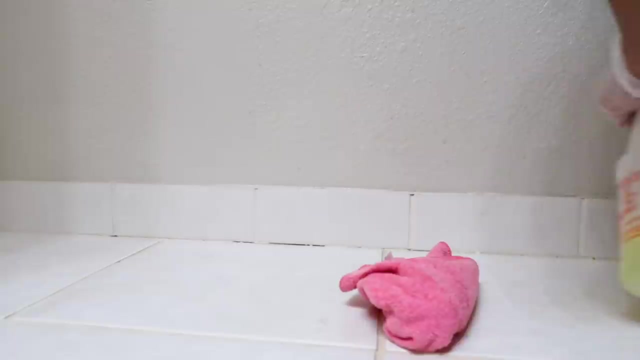 Love, love, love's too deep. You know your love's too deep. You know your love's too deep. I don't have to party To have fun. you see, I got different hobbies And that's all I need. So instead of just dusting it off, 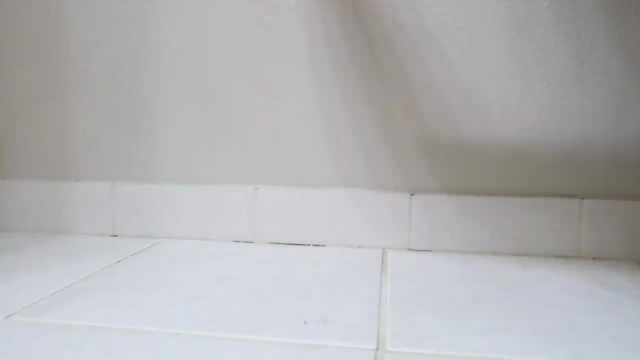 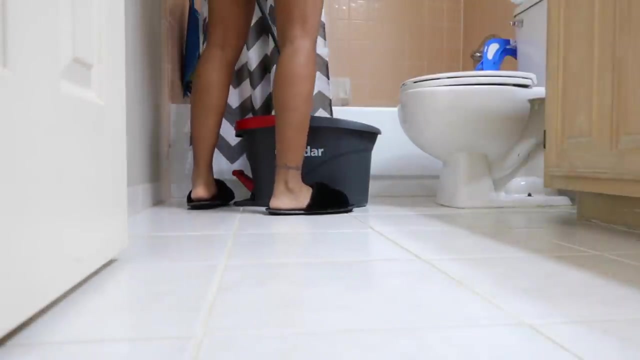 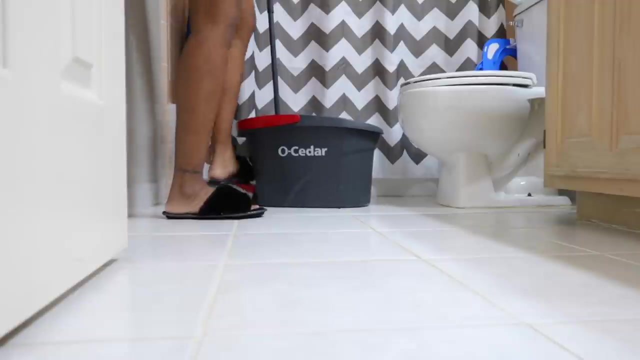 I had to get down and spray some awesome spray To clean off the molding and the wall. Didn't believe it. Mm-hmm, Baby, I'm gonna try, gonna try, gonna try. Work till I die, till I die, till I die, I'm gonna fail and get up. 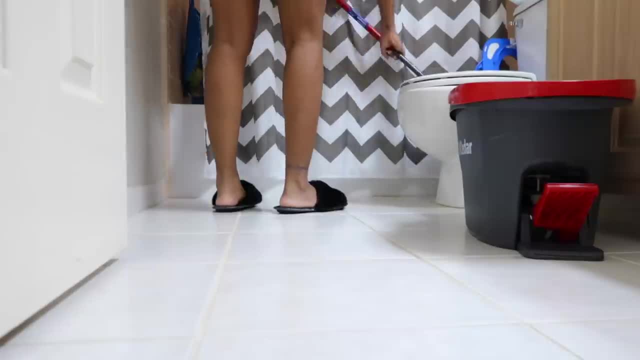 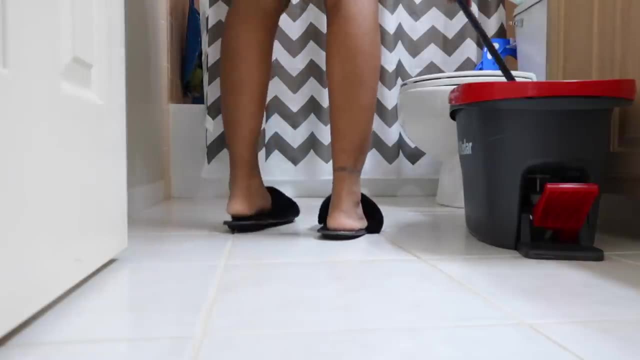 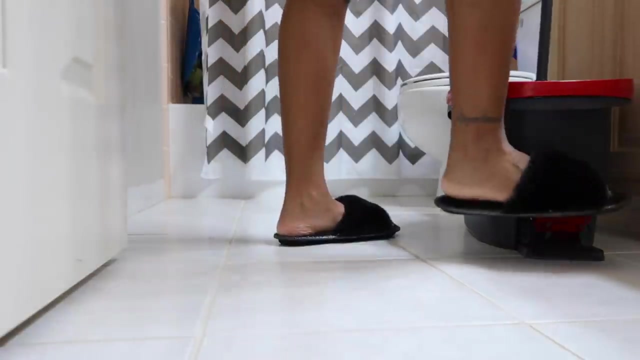 Cause I'm not giving up on my dream. I'm gonna cry, gonna cry, gonna cry, Chasing the highs, yeah, the highs, yeah, the highs. I'm gonna fail and get up, Cause I'm not giving up on my dream. I'm not into drinking. 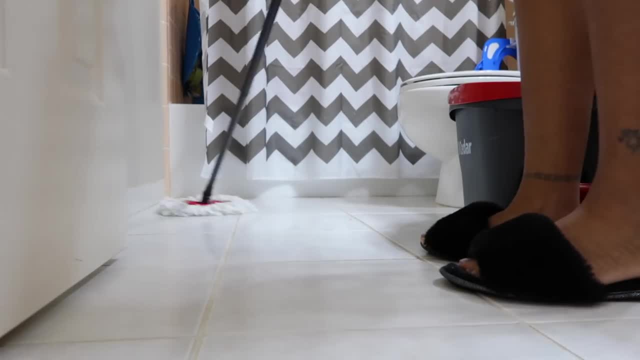 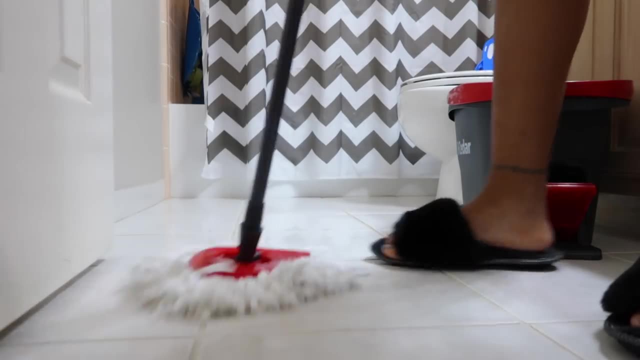 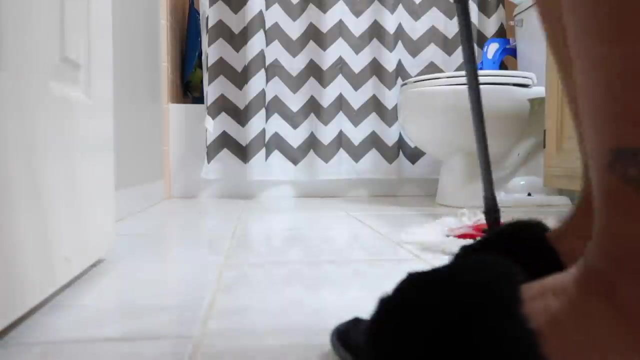 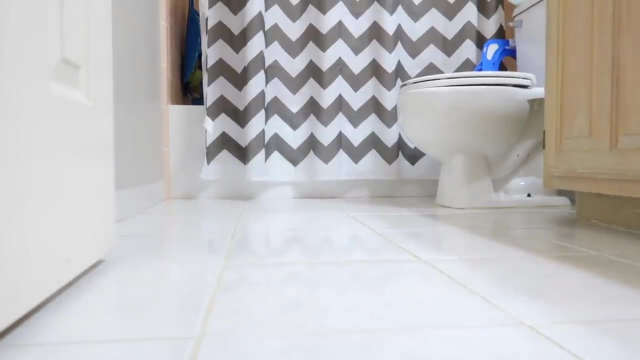 That's just what I do: Wasting time. I'd rather be spending It on working out. Some say I'm too uptight, But I disagree. I wake up and live my dream. Someday soon I'm gonna make it. Yeah, all hard work's gonna be worth it. 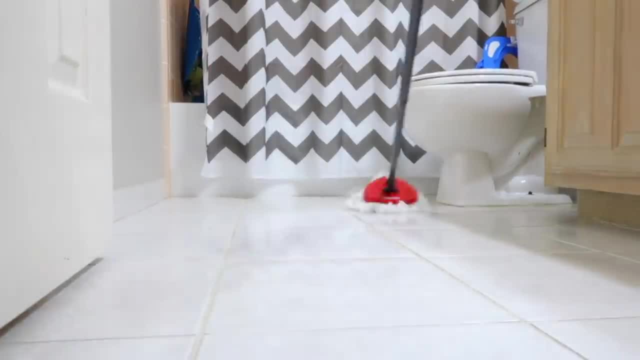 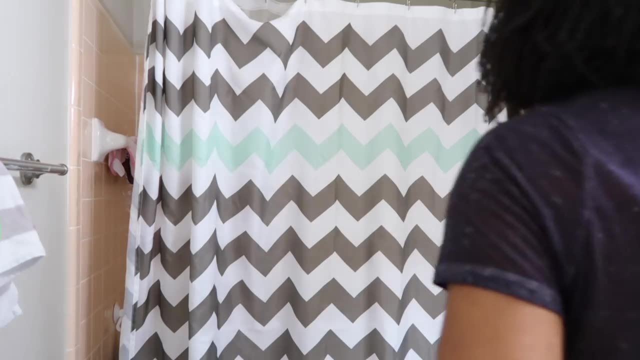 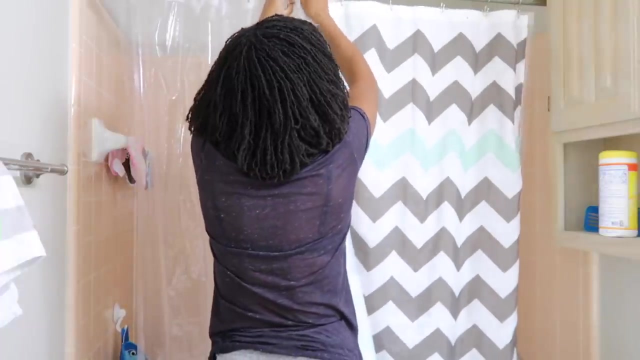 Ooh, everyone who did it Didn't believe it. Mm-hmm, They don't know a thing. I'm gonna try, gonna try, gonna try Work till I die, till I die, till I die. I'm gonna fail and get up, Cause I'm not giving up on my dream. 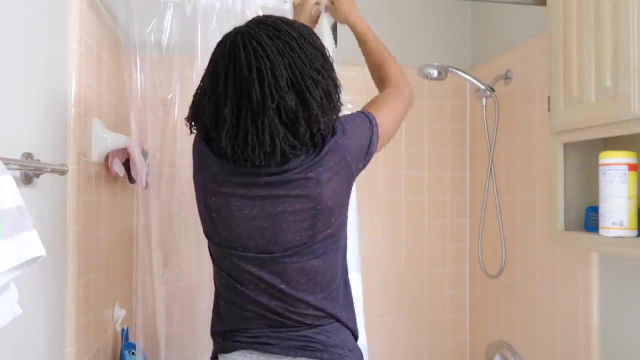 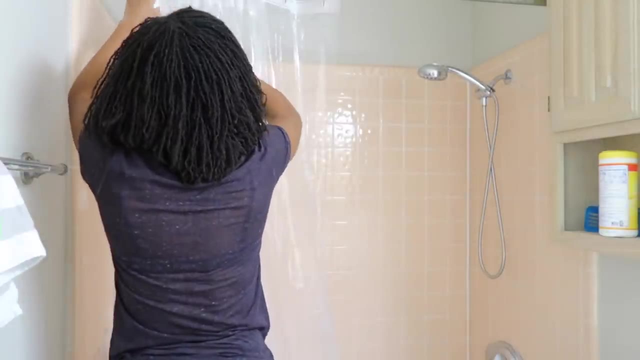 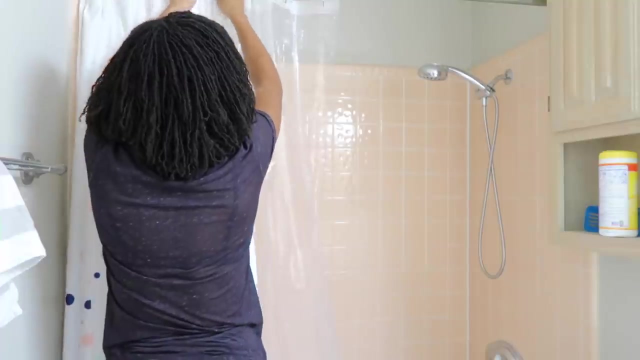 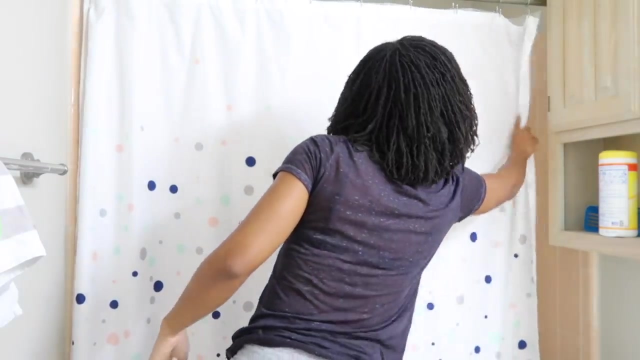 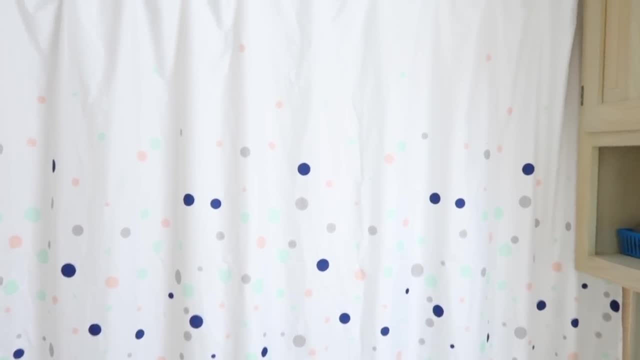 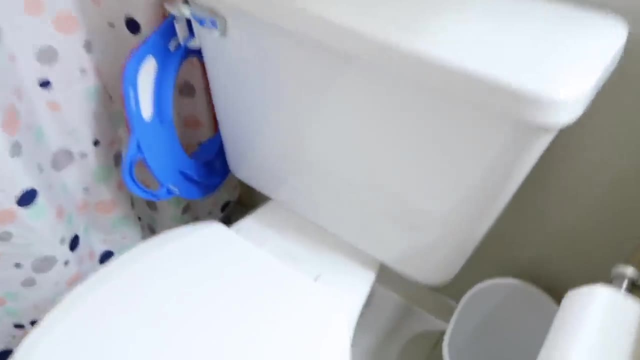 So here's the finished results of the bathroom. I did clean out the tub and the cabinets off camera. The battery died and I was kinda in my groove, so I had to just get the bathroom done. But you guys seen me do that before. 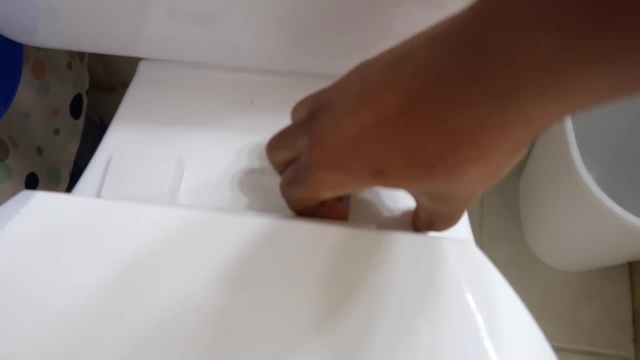 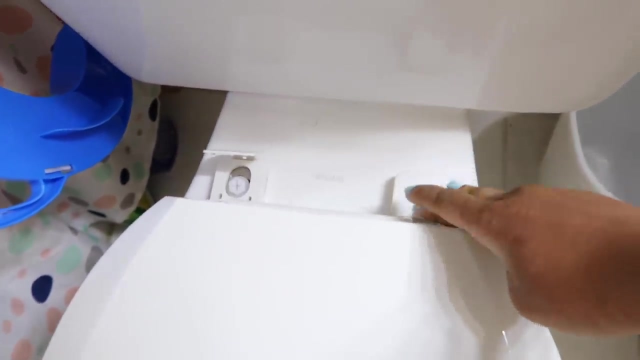 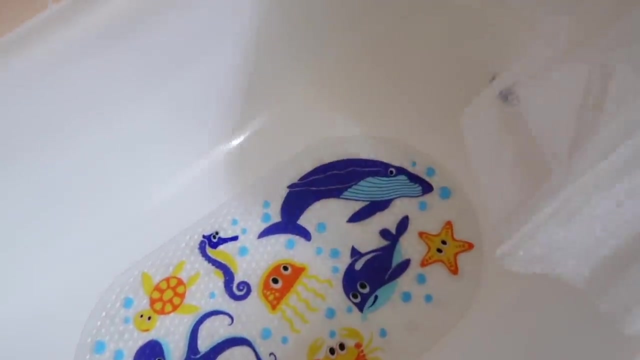 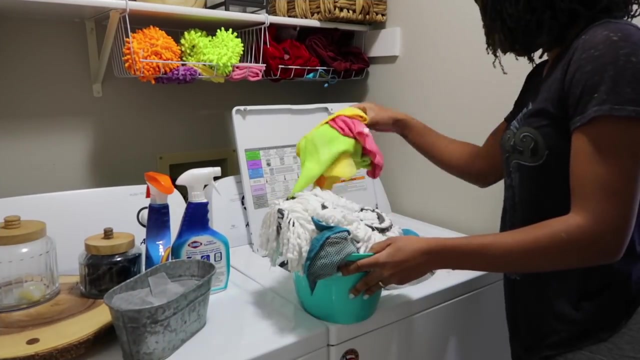 but everything in their bathroom is nice and clean Under the toilet caps are nice and clean now, so I'm gonna be moving right along. Dream dream, dream, dream, dream, Dream dream. I'm not giving up on my dream, So now I'm just going to wash all my cleaning cloths. 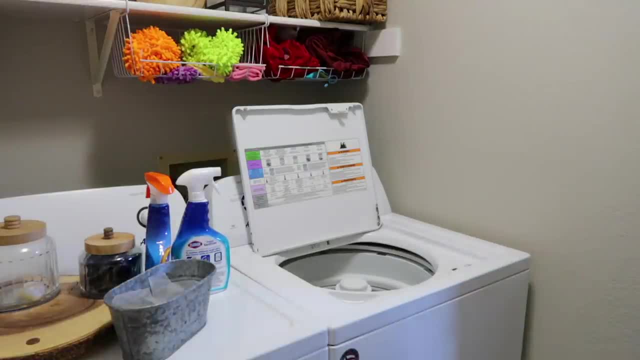 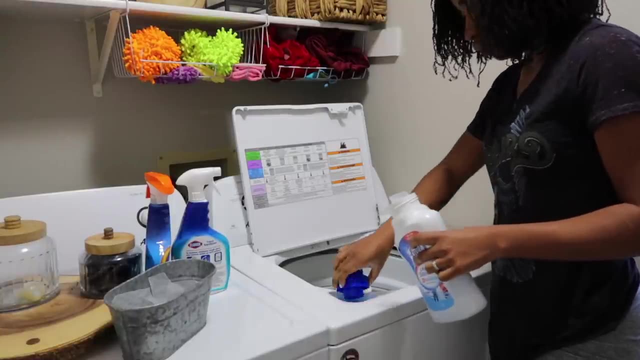 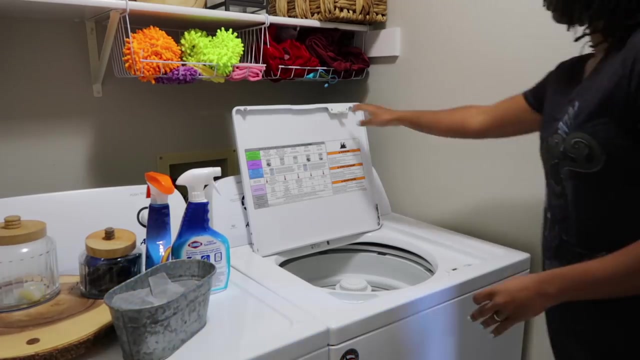 that I use for the day and start that load and then get to folding some laundry. I didn't actually wash any loads of laundry beside this one today, but I had a ton of laundry to fold So I didn't plan on cleaning my bedroom for you guys. 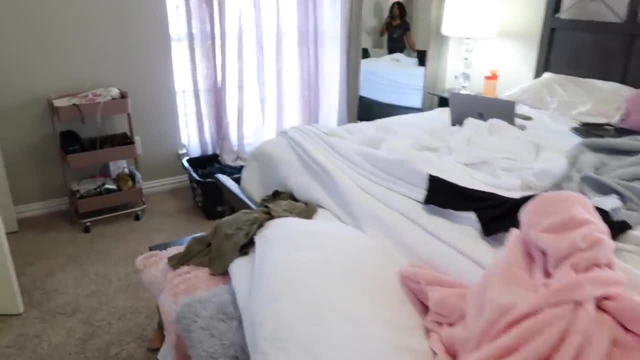 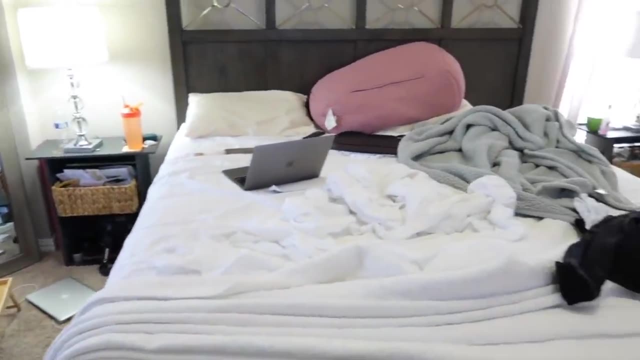 because I just did that. but this is where I wanna do my folding and it's messy again. This is why I say my daughter got it honestly. But that's okay. I'm gonna use a little YouTube magic and clean my room real quick. 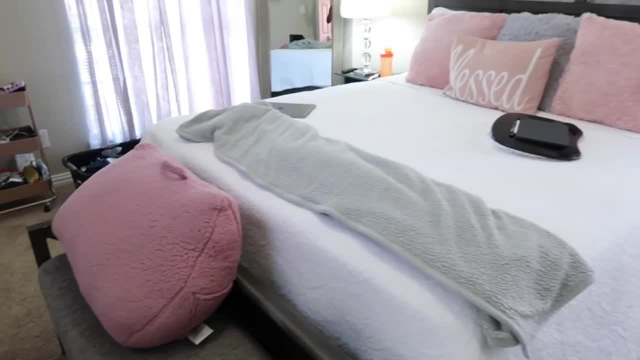 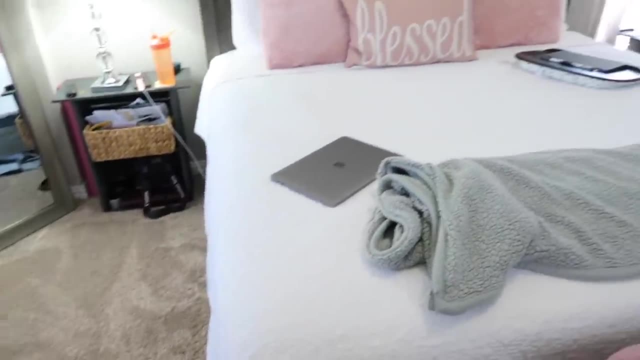 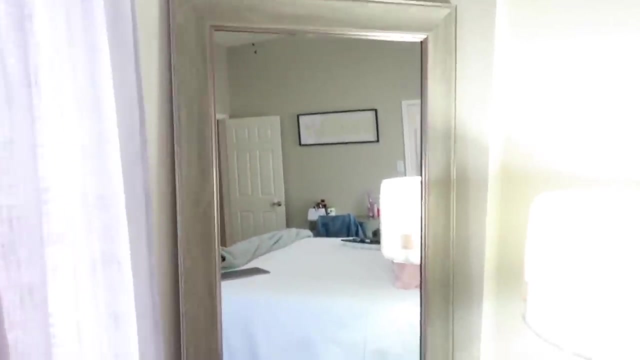 Voila, there we go. So now I have a clean, organized space to fold all my laundry, And here is a new addition to my room. I did add a full length mirror over here. I've always wanted one, kinda just getting ready, in my room. 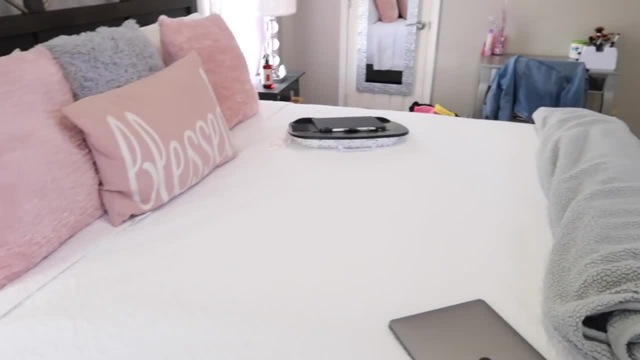 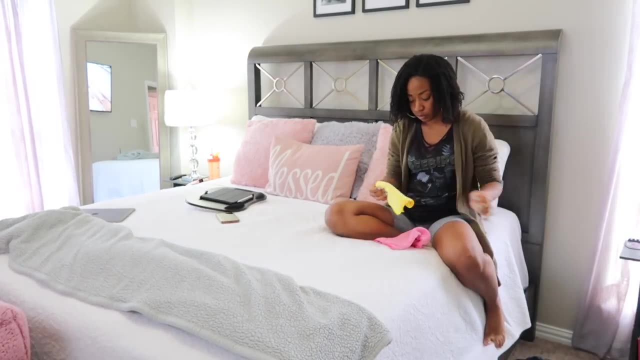 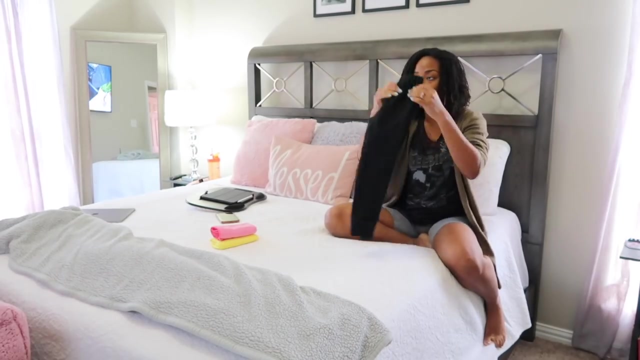 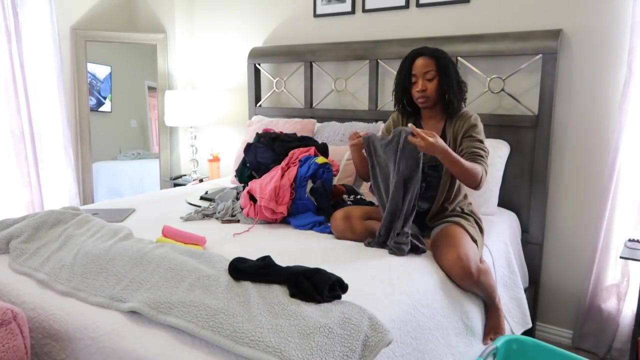 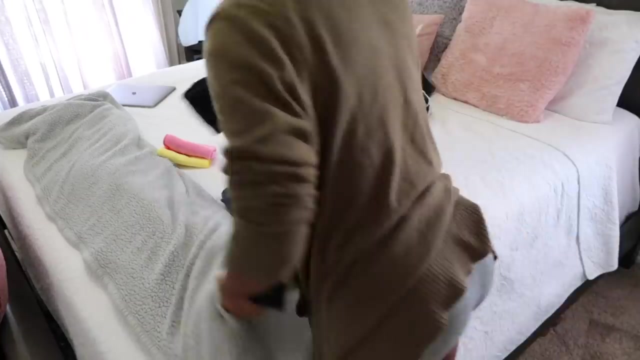 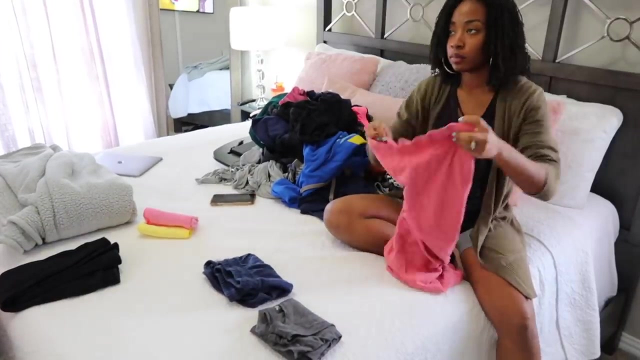 so I'm loving this mirror, and it was only $60 from Walmart. I don't feel like I'm gonna need it today, but it is worth putting out this mirror. So there you go. all you gotta do is take your card and you're done. 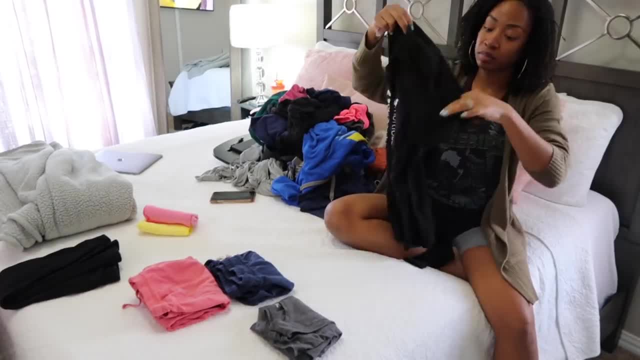 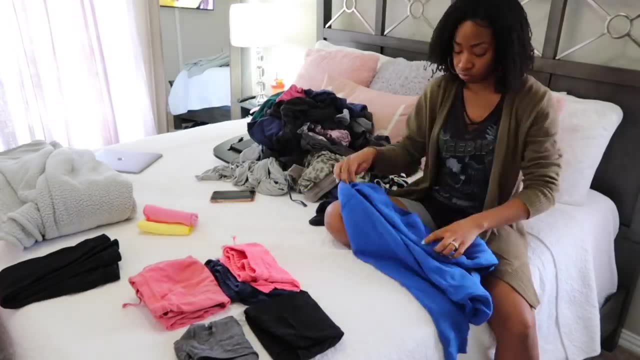 Lastly, I put the laundry in this box like that, Then in the closet, I put all my laundry in there. So that's the bathroom. These are the other living rooms that I'm gonna use for the living room And then. 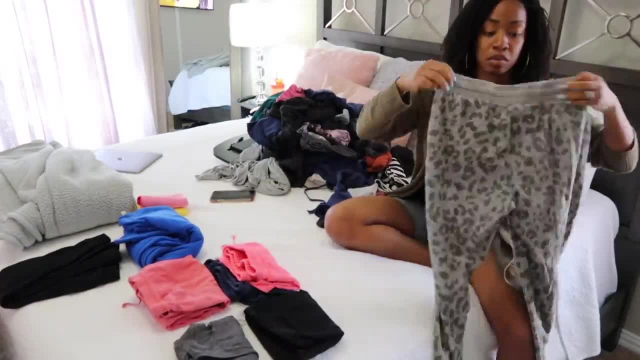 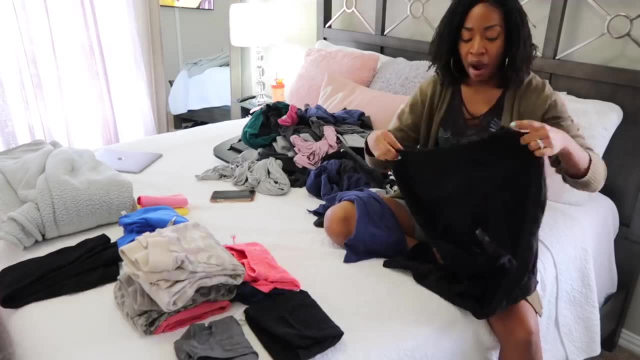 the rooms that I already have. in this room, I also put up windows and curtains, So this is where I put my laundry in. I'm slipping in too deep. This is what I need. Better off, We're getting close. Keep calling each other friends. 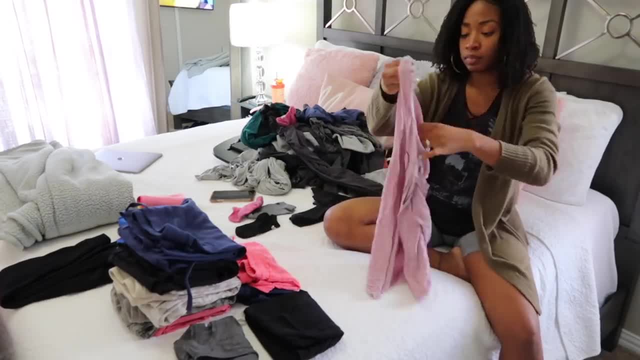 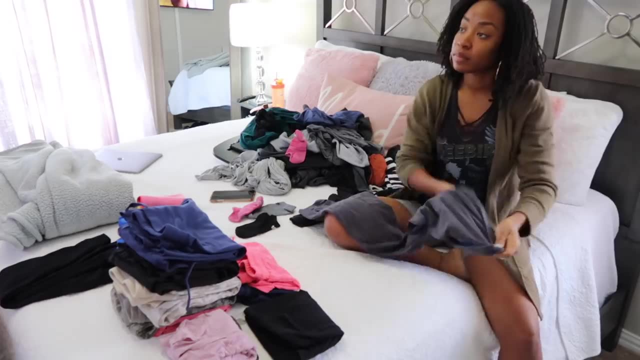 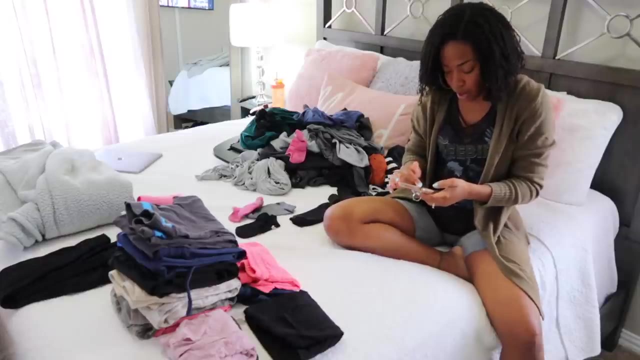 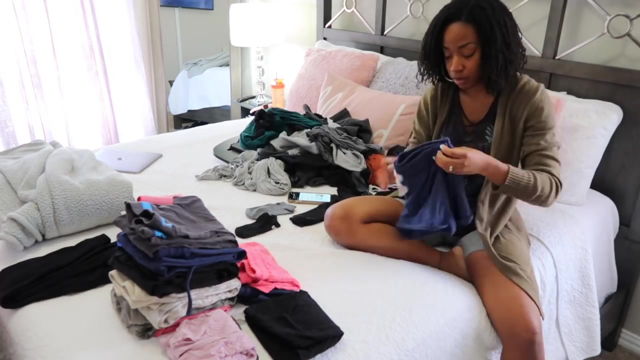 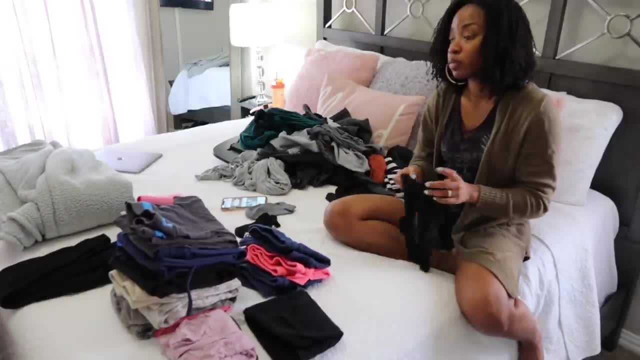 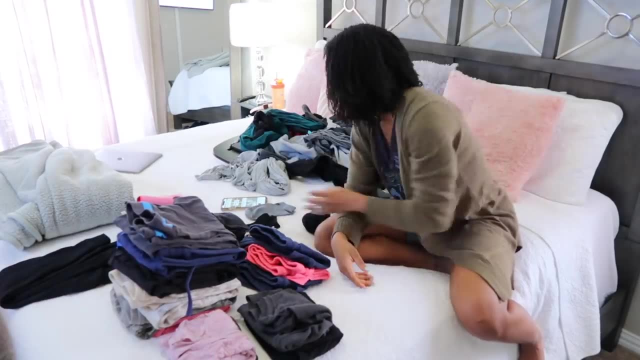 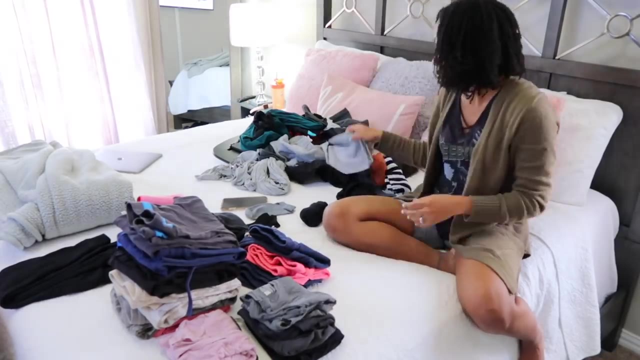 Calling us friends, Calling us friends. I'm by myself, but never alone. I got my friends when I'm on my own. Calling us friends, Calling us friends, Calling us friends. So I'm ending the video with a little bit of laundry folding motivation. I'm sure everyone has. 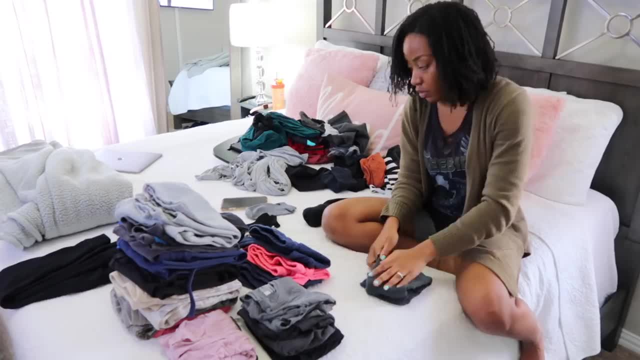 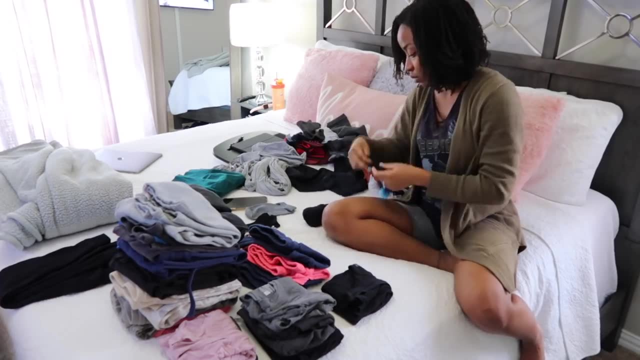 A load of laundry that they could get to right now. So if you do grab that load of laundry as you finish watching this video and let's get that done- Can't guarantee you'll get it put away, but at least you can get a load folded. 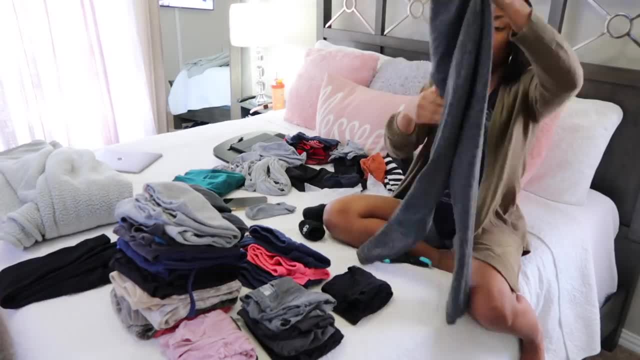 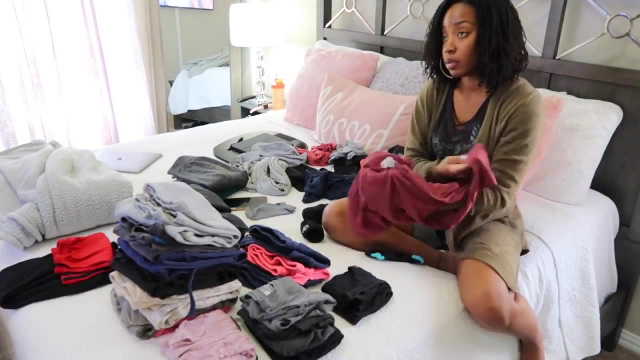 Thank you so much for watching it. If you're still here at this point, you are the real MVP. I appreciate you guys for supporting my channel. I'm really grateful for that, because you could be watching anyone on the internet and you chose to watch me.